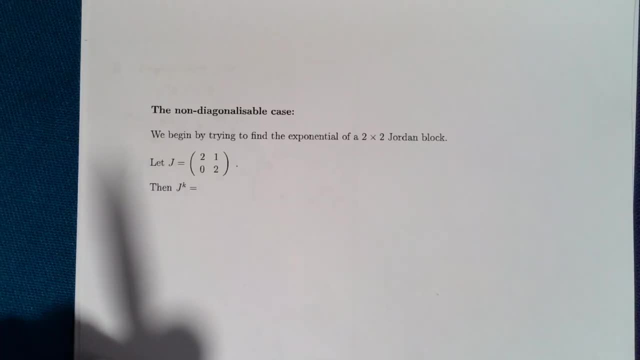 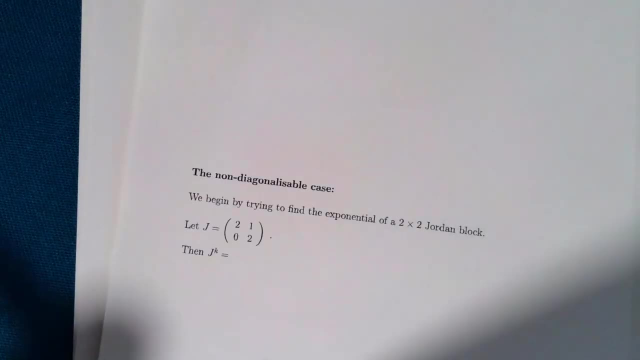 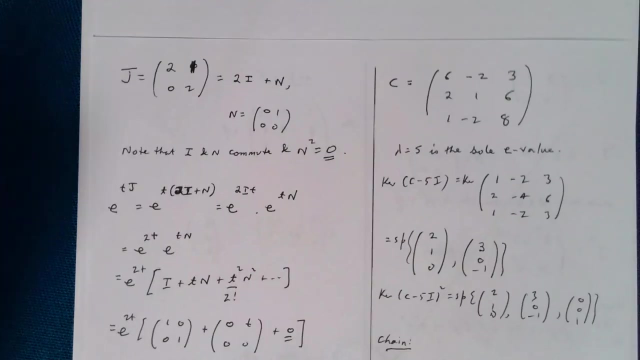 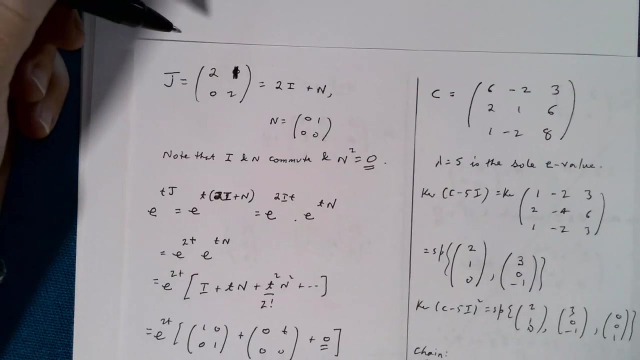 the exponential matrix looks like. So we will calculate that here. In fact, I'm going to calculate not just J to the K. I'm going to work out E to the, I'm going to work out the exponential of this one. So here's our Jordan block And it's just a little two by two matrix here, So I can. 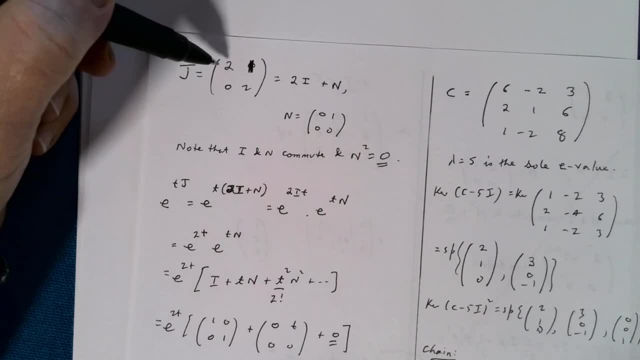 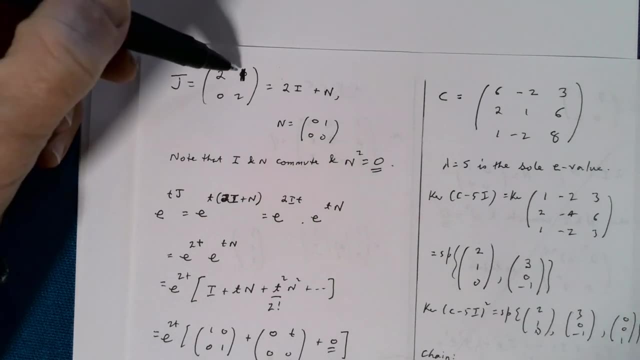 write this. I can split this up, as we've done before, into twice the identity matrix to take care of these two, twos, plus a little n matrix, a nilpotent matrix with just zeros and a one there. Now, of course, i and n commute because i is the identity And n squared if you square. 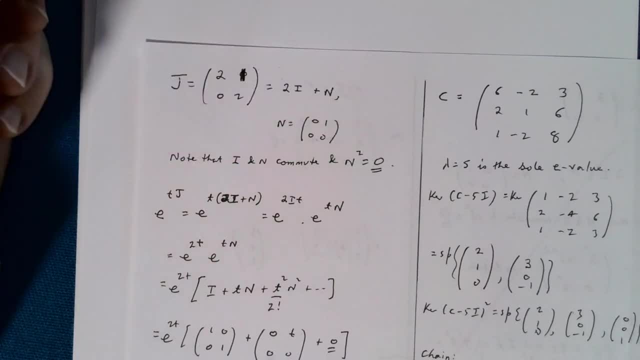 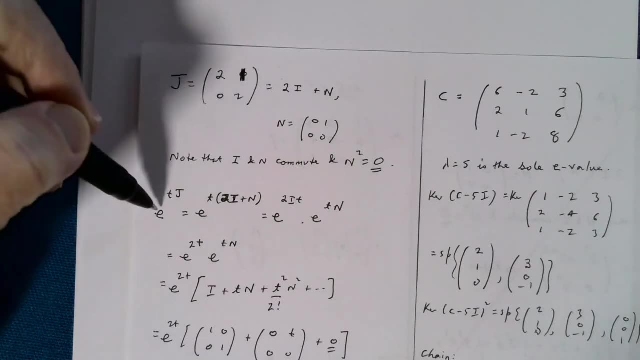 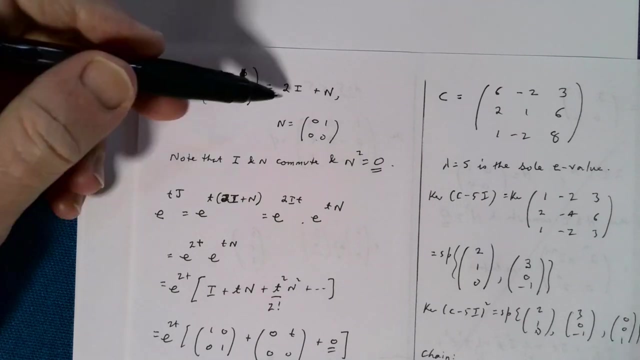 this matrix, you just get the zero matrix. So again, I'm going to go back to the definition of what we mean by an exponential. Before I do that, I'm just going to write this: either the Jt or either the Tj. here I'm going to write the J as 2i plus n And I'm then going 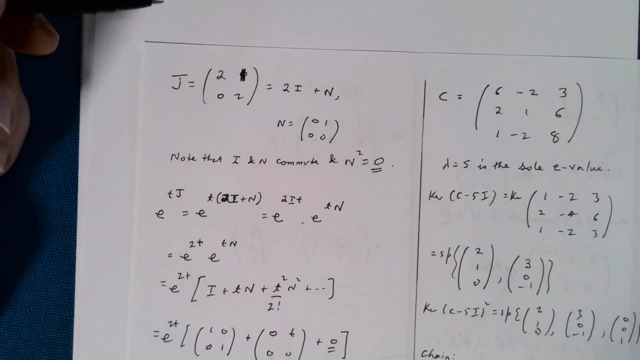 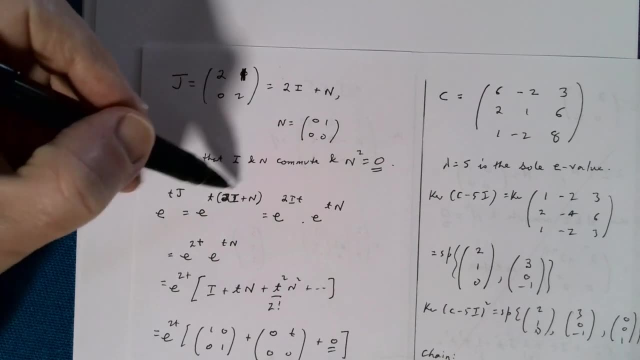 to use the, The, The, The, The index laws here that these two things are matrices, And so I'm going to split this up into either the 2it times, either the Tn, And the point is that either the 2it, if you. 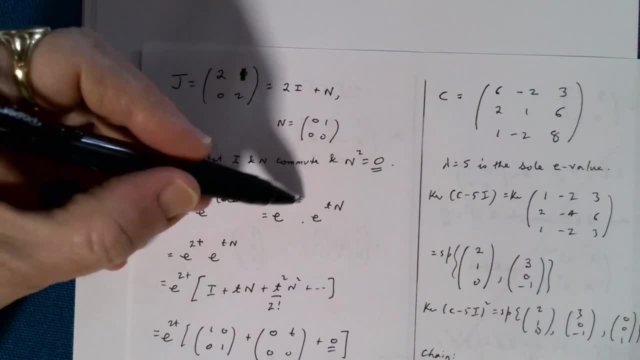 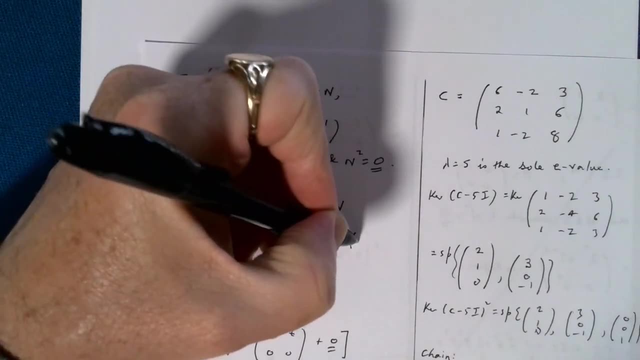 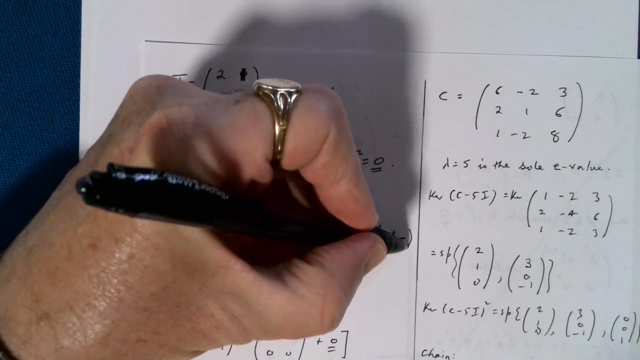 multiply. If you write this out as a series, then you just get either the it times the identity matrix. So I'm really using the fact here that either the 2it is really either the 2t or the identity matrix, And when you multiply the identity matrix times anything. you just 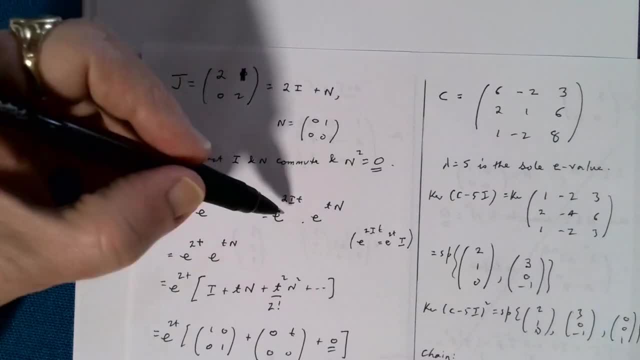 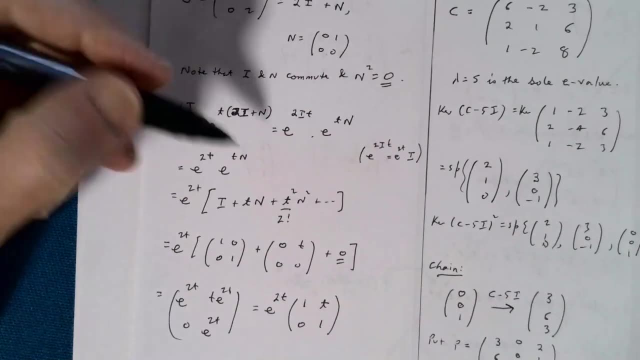 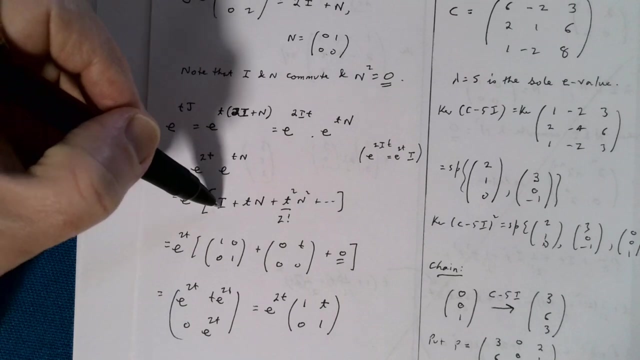 get back what you started with. So this product here is just either the 2t times either the Tn. Now, the point is now n is a nilpotent matrix, And so when I write down the Taylor expansion for this, I'm just going to get i plus Tn plus T, squared on 2 factorial n. 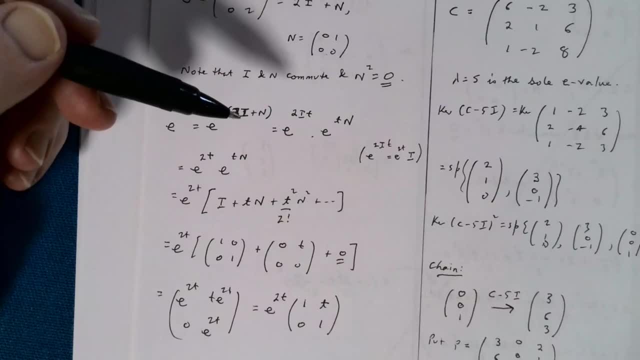 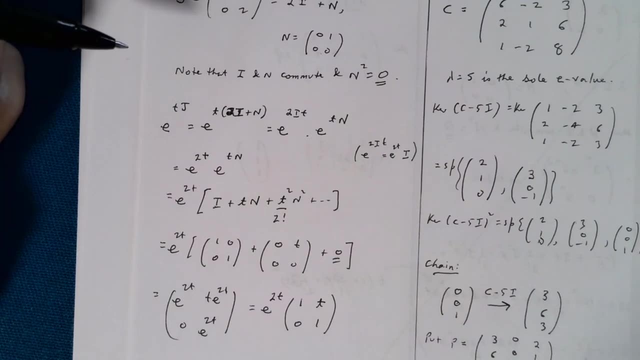 squared plus and so on, But of course n squared is the, The N squared is the zero matrix, and all of the higher powers of n are going to be zero matrices, And so all I end up with then is just the identity plus T times n, which is this matrix. 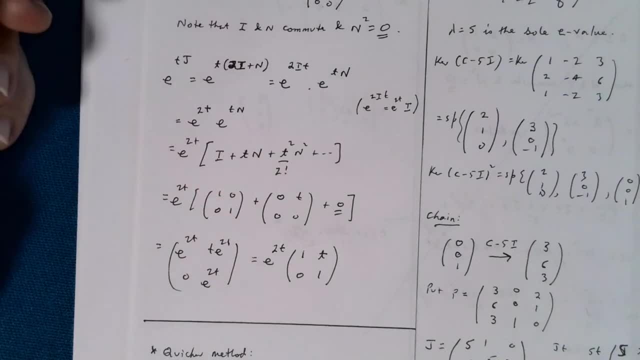 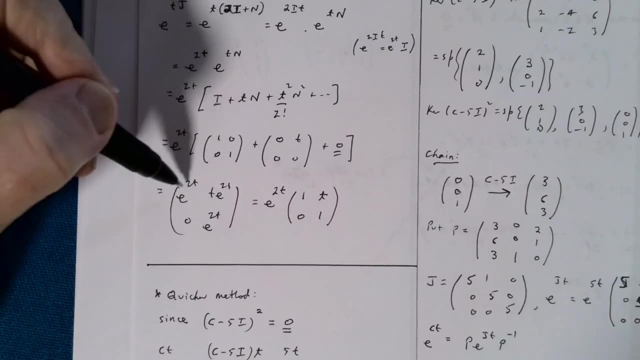 plus, I'm going to get a whole pile of zero matrices And simplifying this, I get either the- I just enjoy the shape of this. We get either the 2t, either the 2t on the nine diagonal, as we might expect, But on the off diagonal. 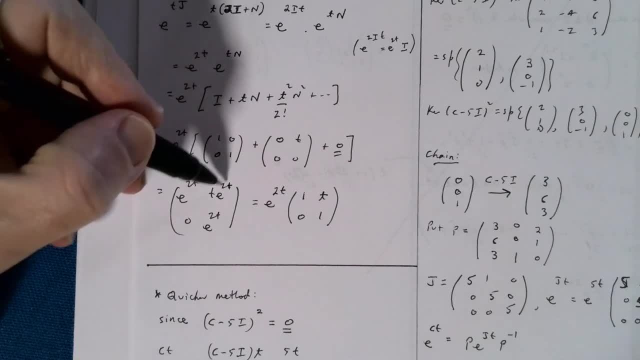 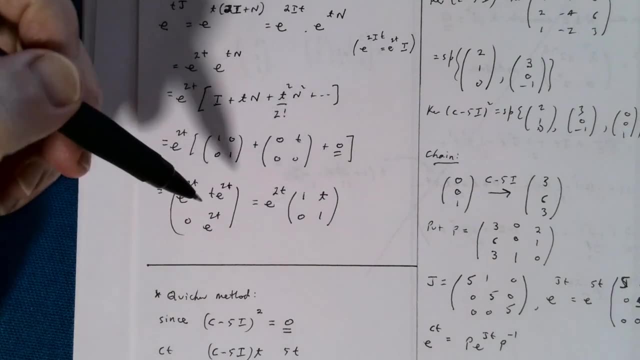 So, Yeah, Yeah, entry here. I get t, e to the 2t and I could also write that as e to the 2t times: 1 t 0, 1. so there is our formula for e to the jt. we've found the exponential of a simple 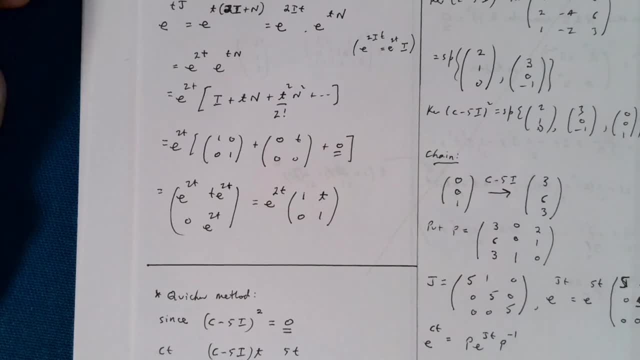 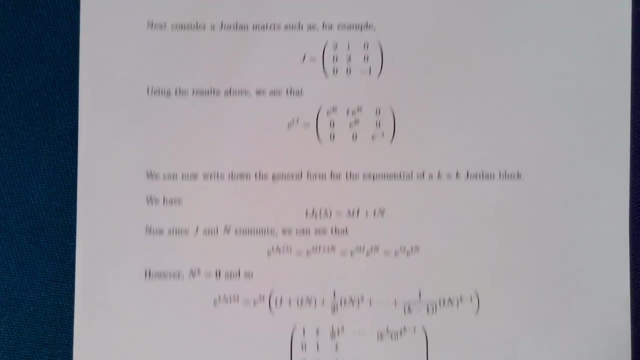 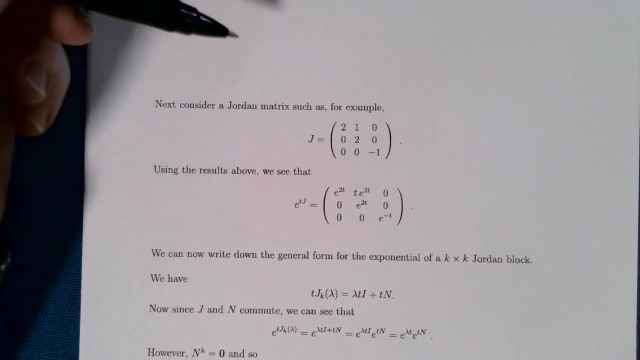 2 by 2 matrix. well, we move up a little bit, try and pattern match here and see what happens for higher degree ones, and without going through all the calculations, I'm now going to just look at a slightly more complicated one. so here's a Jordan matrix. here now this Jordan matrix. 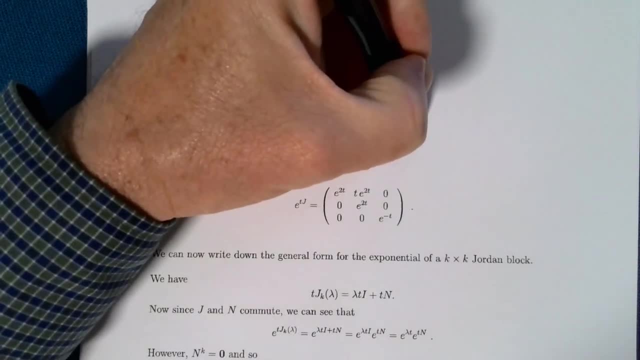 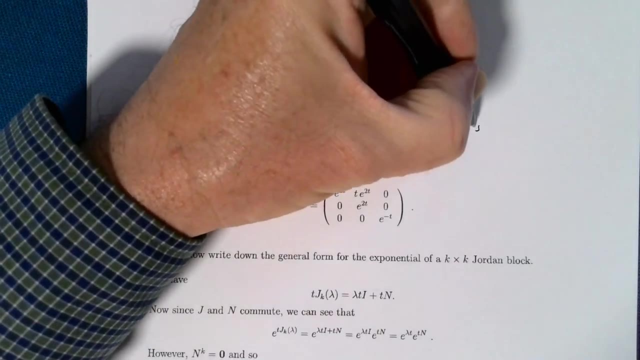 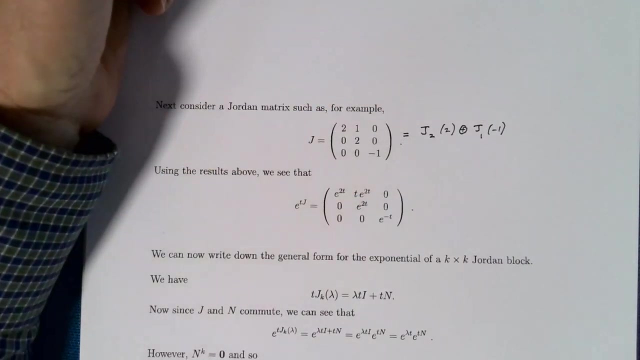 is going to be equal to its j2, 2 by 2 block based on the eigenvalue 2, and then direct sum j1 based on the eigenvalue minus 1. so we get direct sum of two Jordan blocks here, and I can use exactly what I've done. 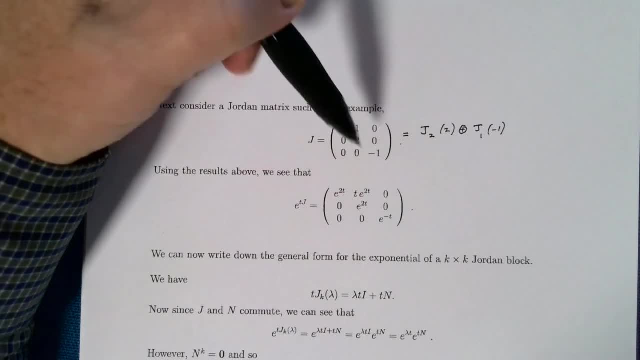 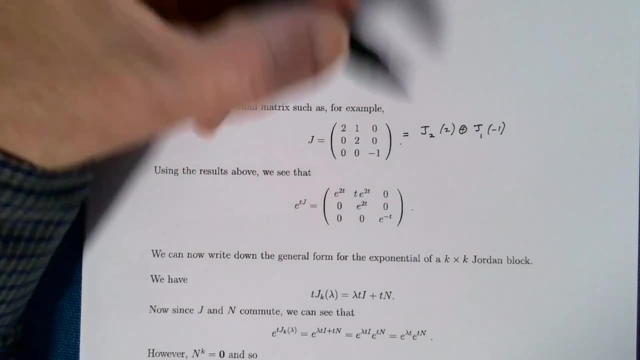 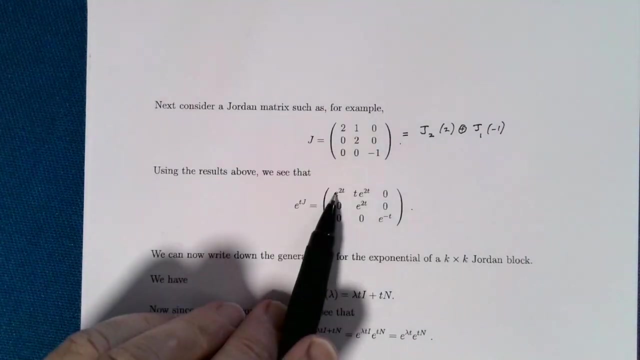 before. we've already found the exponential of this one and we know that this one is just a simple diagonal matrix that's got one entry in it, so we would expect that the exponential of this just looks like either the 2t, either the 2t t, either the 2t with 0s. 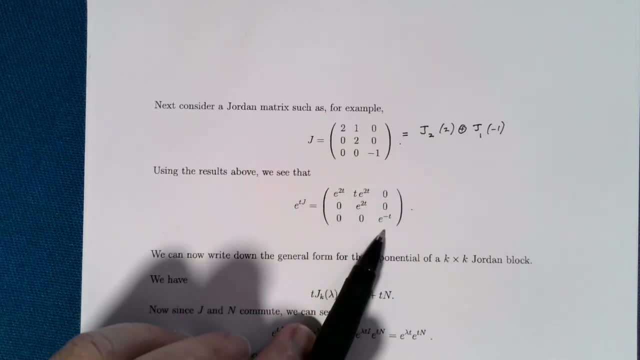 all around and a nice little e to the minus t in here. well, I'm just going to write down now the general form. I'm going to just do what I did before in a more general setting and write down the following: if I've got a Jordan block of, 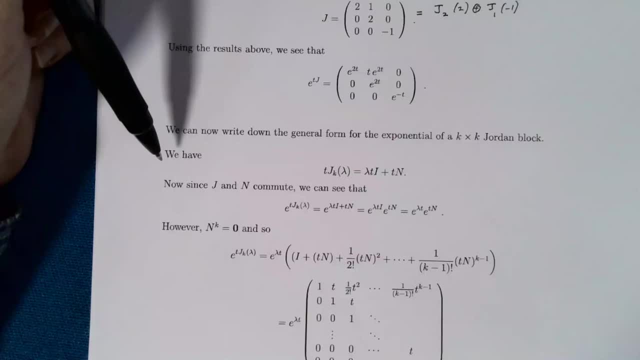 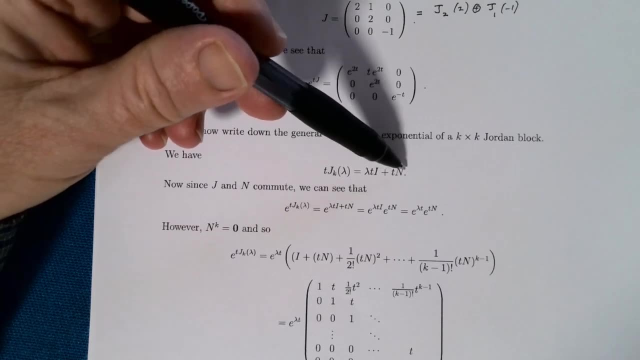 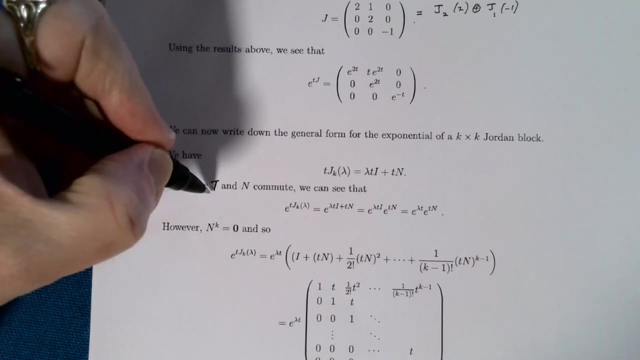 k by k Jordan block. and once again I'm going to split this up into lambda I, lambda t, i plus t, n, where n is this nil potent matrix and the i and n commute should be i and n. so these two matrices, because this is an identity these commute with. 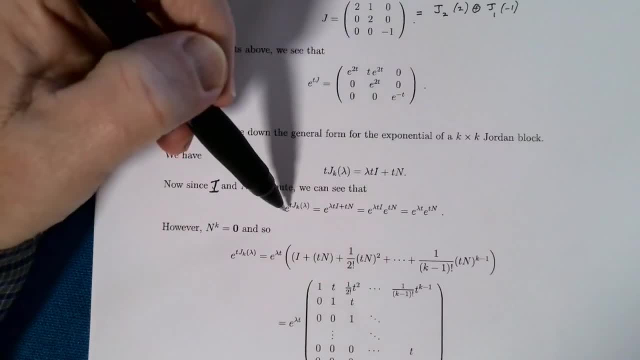 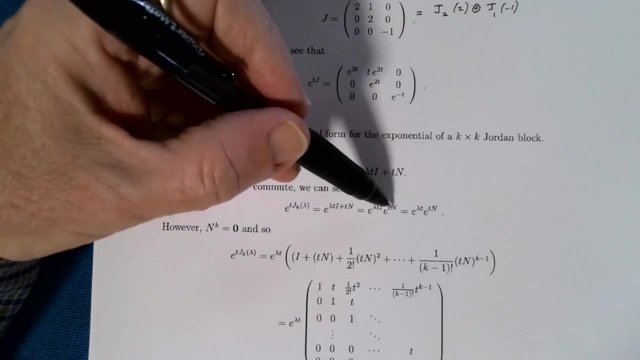 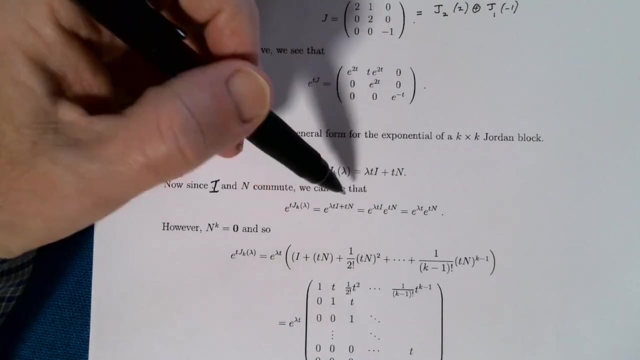 each other, and so once again, I can write either the T, either the JT is just lambda TI plus TN. I can split this up only because these two matrices commute. in general you can't do this. this is only true here, because the matrices commute, and again this thing here is just either the lambda T times the identity. 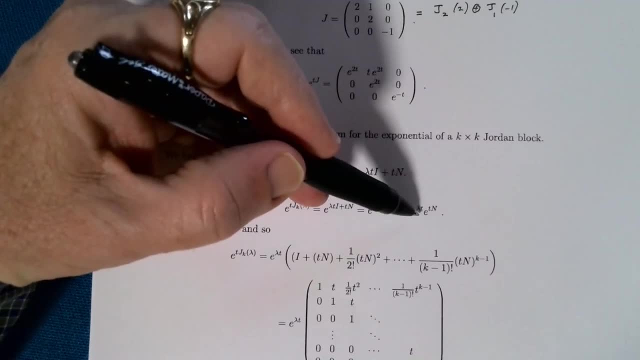 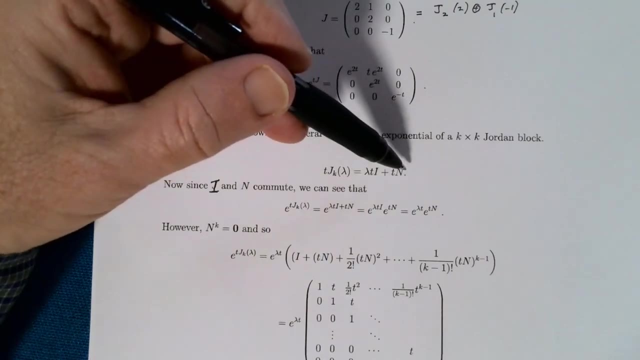 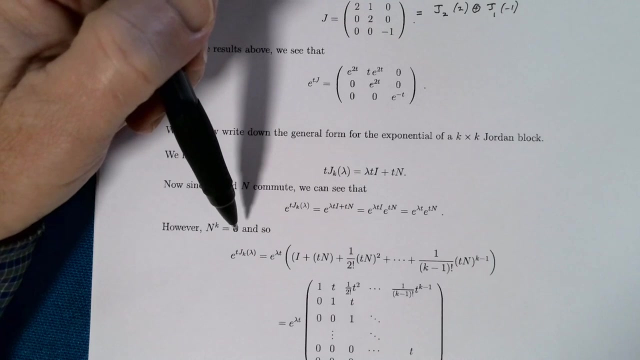 matrix and when you multiply the identity times, either the TN, you just get into the TN. now our N is a nil potent matrix and it's a K by K block. so N to the K is the zero matrix, and so I can expand out either the TN as its Taylor series, but it's going to stop at this. 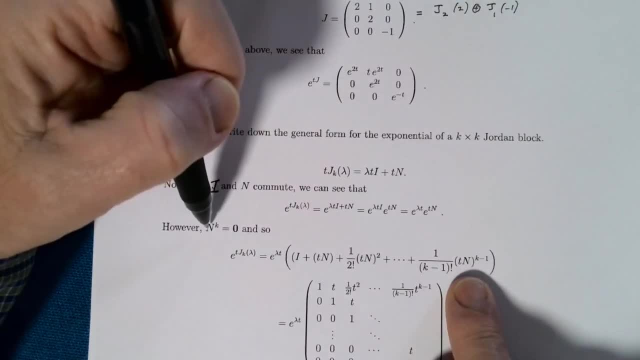 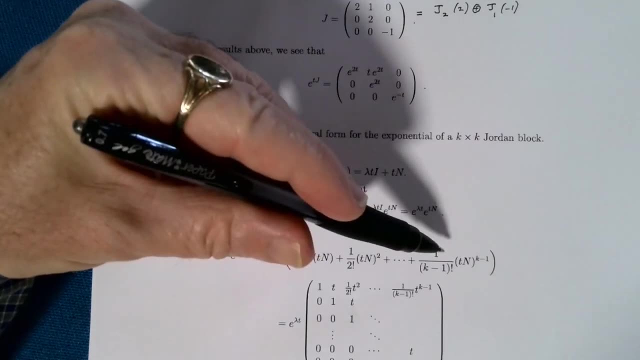 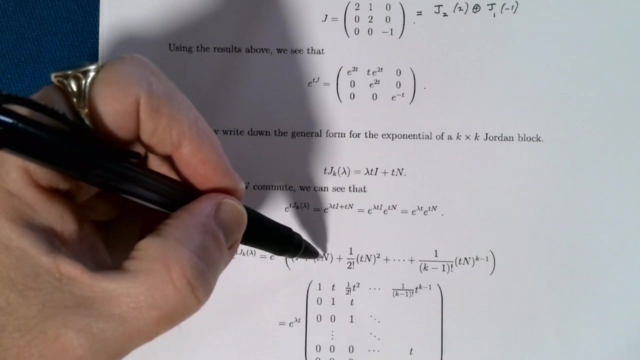 point, because once I go any further, I'm going to get a whole pile of zero matrices coming out the side here and now I'm just going to write down what this looks like. so this is going to have ones on the main diagonal and I'm going to get a T. I'm then going to get when you square this, if you look at N squared- 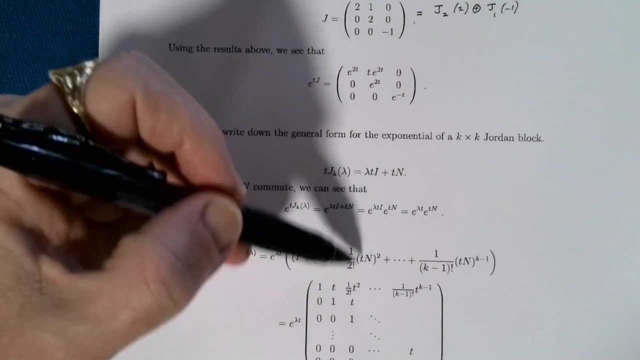 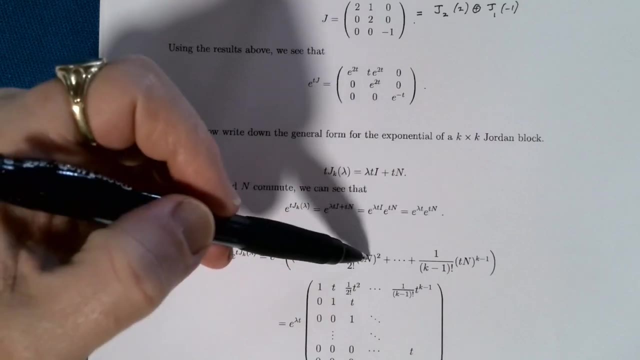 that pushes the one further across. so I'm going to get one on two factorial T squared, and so on. the ones get every higher power of N that I take, the ones get pushed further across, and so the next term here will be one over three factorial T cubed, and at the end I'm 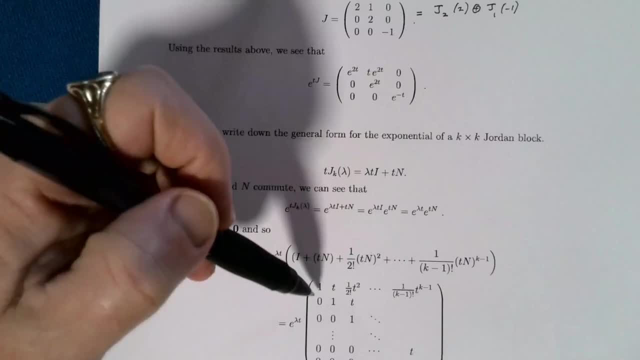 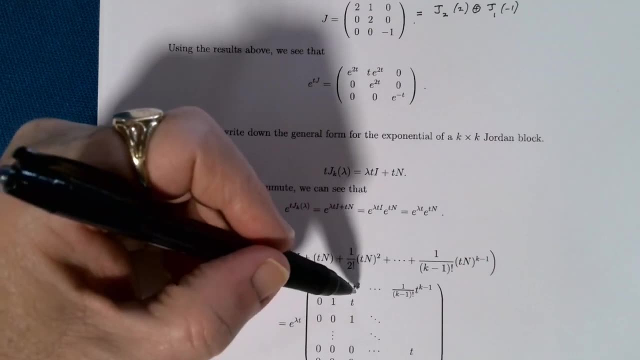 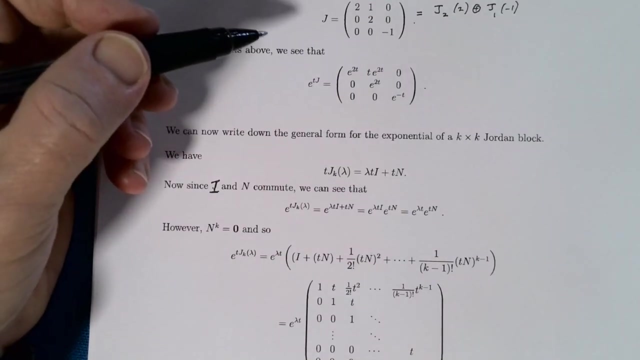 going to get this one here and the same is going to happen here. so I'm going to get one over three to happen across every row here. so this will be one t. this next entry is one. two factorial t, squared, and so on and so on all the way down. so that's going to be the basic shape of the. so 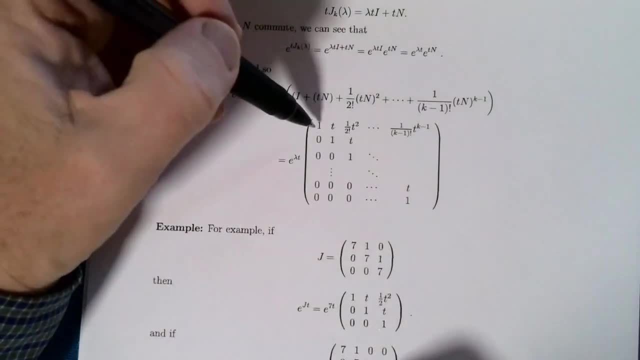 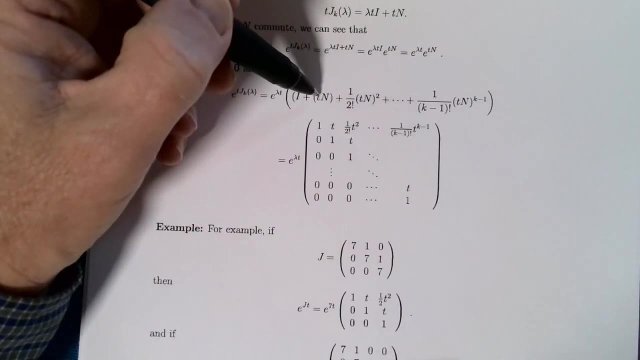 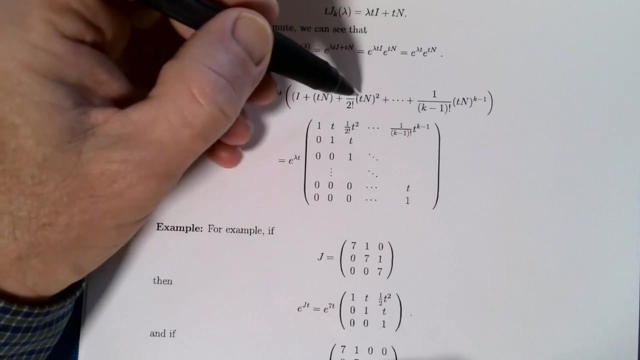 that's going to be the basic shape of the matrix. when we expand this out we'll get ones down the main diagonal, from the i and tn is going to give me t's down the main diagonal, down the off diagonal, n squared pushes the one further out. so this term is going to occur on this diagonal further out. 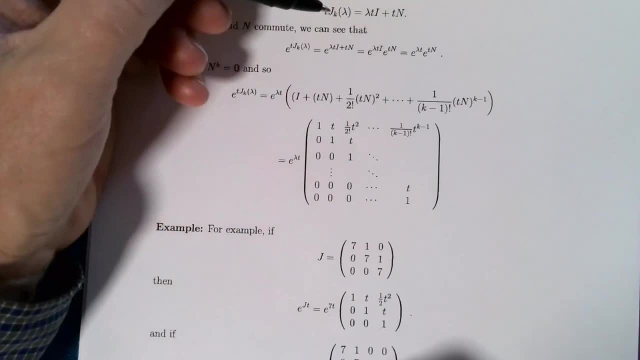 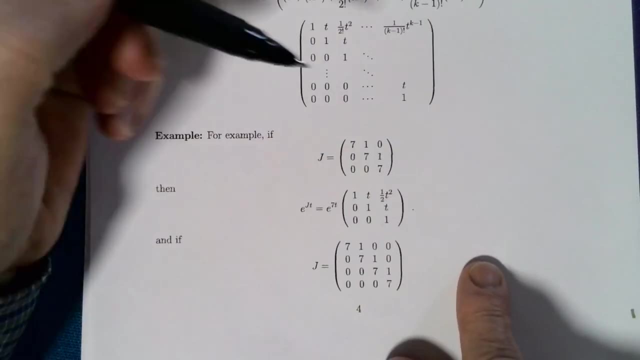 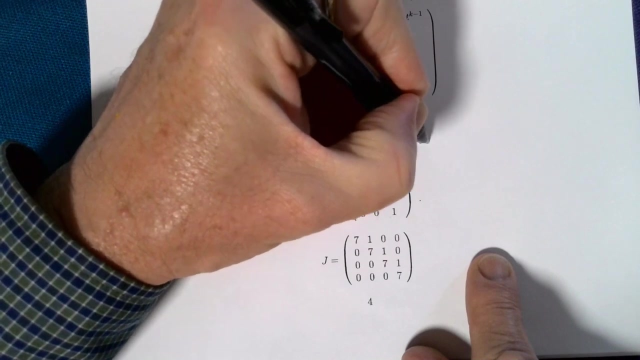 n cubed pushes the one further out again and so on. so just seen by example here, if i take this one here, i've got this jordan block here. this is um a three block block based on seven. so this is a jordan block of size three, based on eigenvalue seven. and if i take the exponential of this then 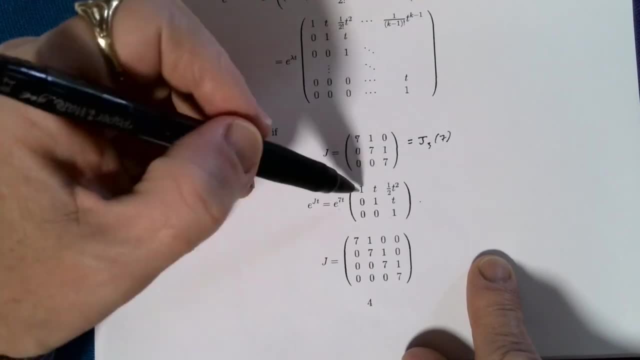 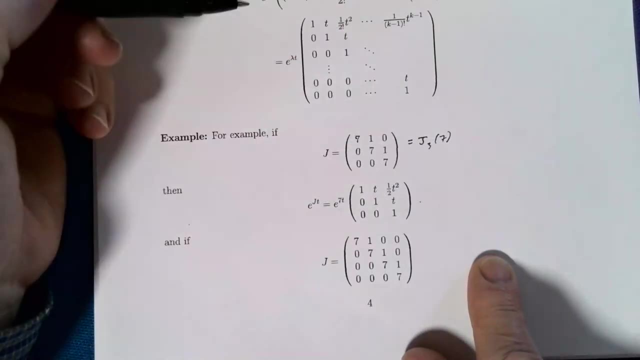 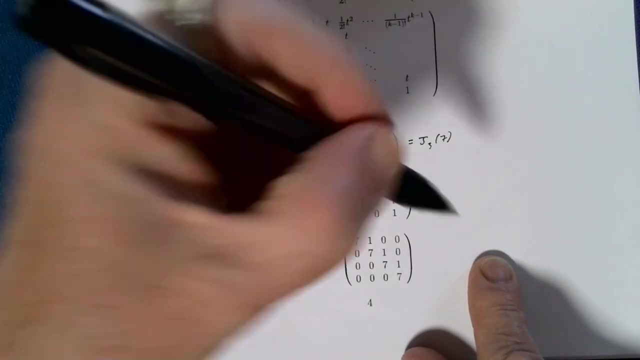 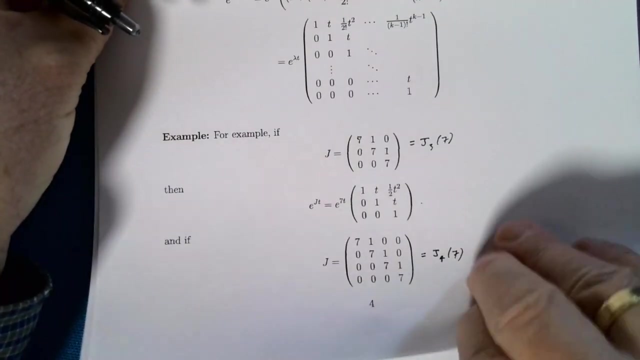 it's just e to the seven t. i get ones down the main diagonal, t's on the off diagonal and one on two factorial, which is just two t squared on the on the top here. similarly, if i take a big four by four jordan block, so this is a jordan block of size four based on seven, and i exponentiate that i work out either. 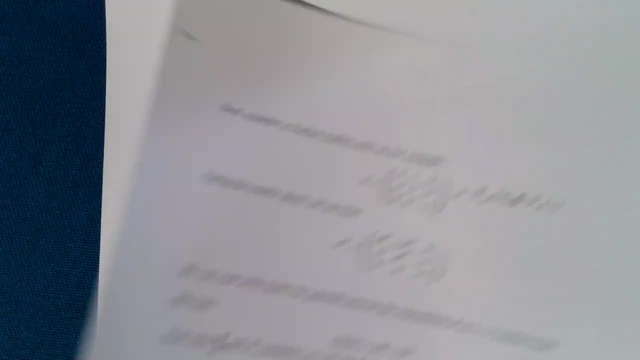 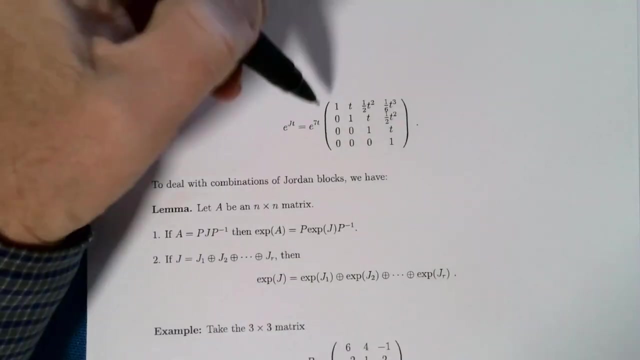 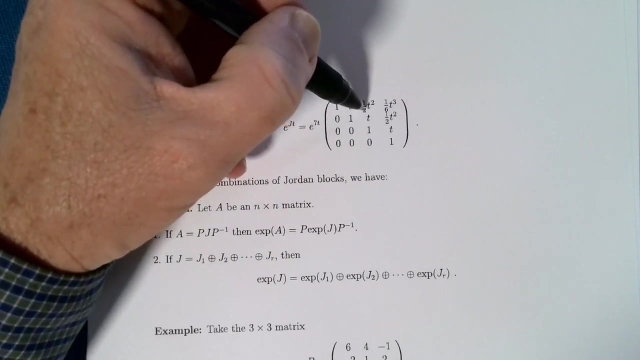 the j t, then i'm going to get something like this one one i'm going to get um. so either the j? t will be just e to the seven t, one's on the main diagonal, t's on the off diagonal, one over two factorial. two factorial is two t squared on the next off. 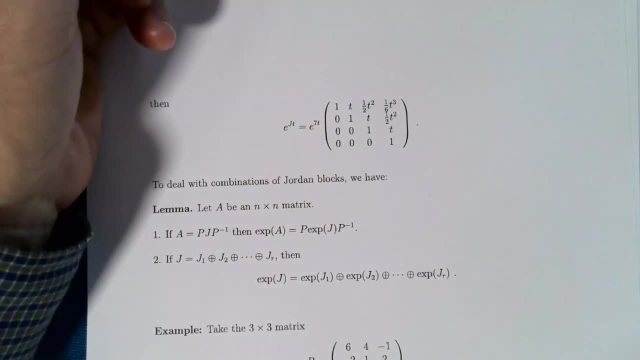 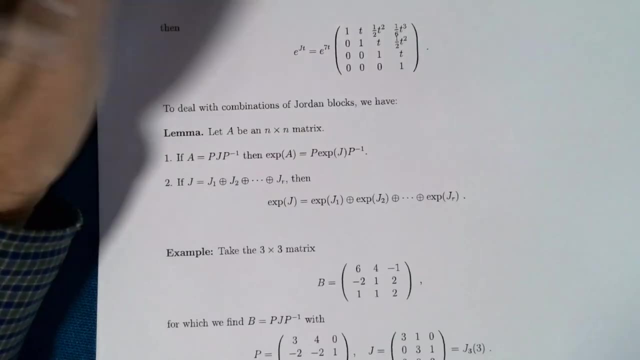 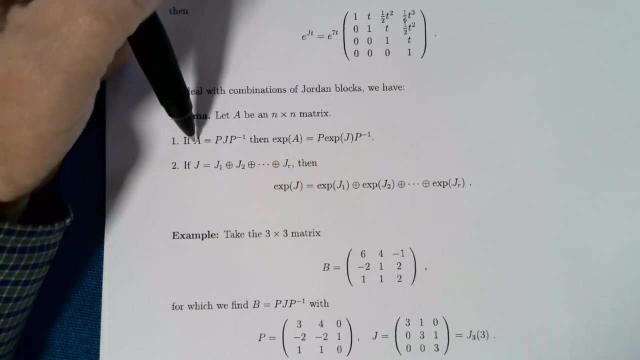 diagonal and then three factorial is six, so i get one on six t cubed. now to deal with combinations of jordan blocks, we simply um have the following little lemma: we've got an n by n matrix, so a will have a jordan form. so i can write a as p, j p inverse and then uh, e to the a, then is p, e to the j p. 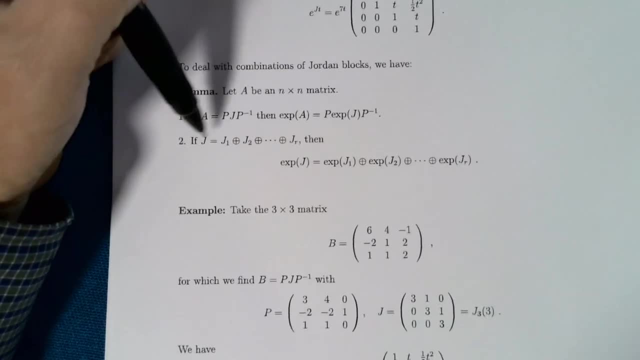 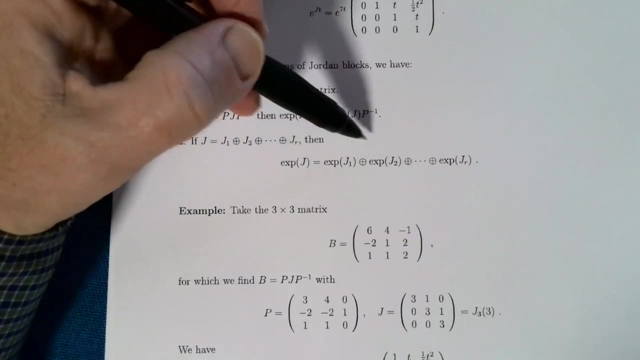 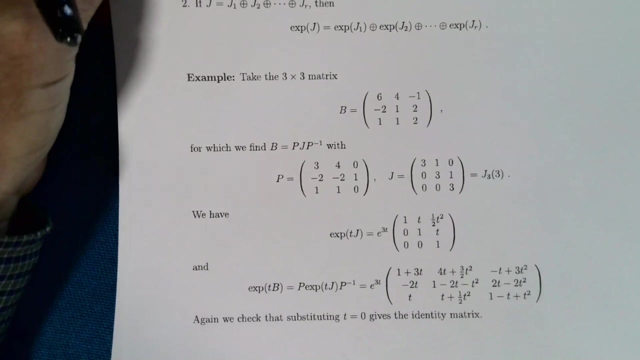 inverse, and if j is a direct sum of jordan blocks, then e to the j is just the direct sum of the exponentials of each of the jordan blocks, which is very nice. so again, just a quick example. here we take a three by three matrix. 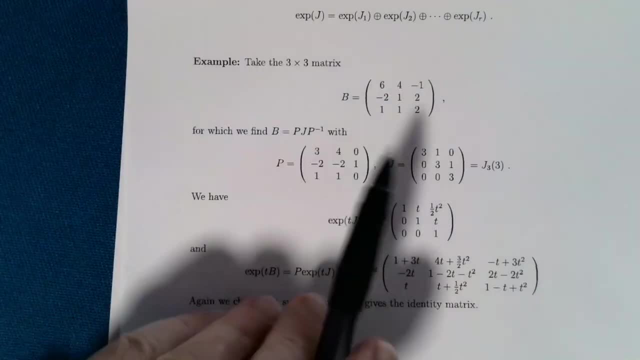 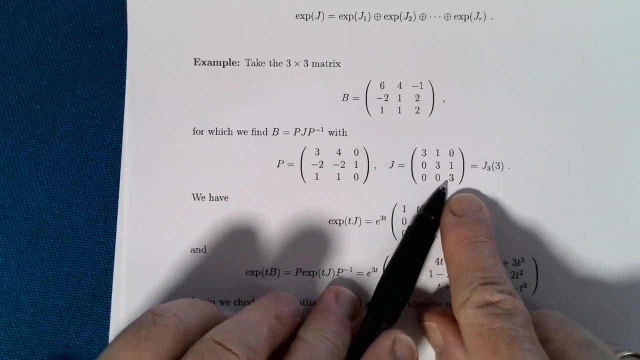 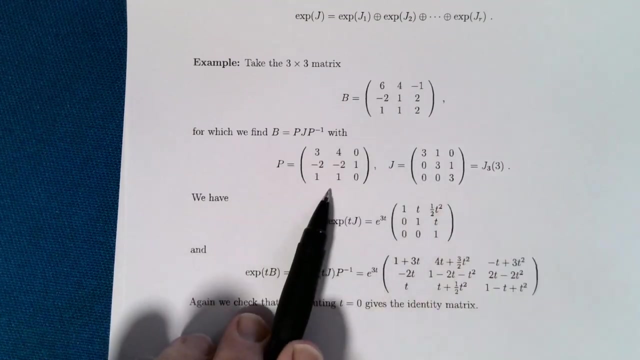 we do all the usual analysis on this, we find that this um has a jordan form that looks like this one. so the eigenvalue is three. so it's only got one eigenvalue. it's got geometric multiplicity one, algebraic multiplicity three and the change of basis matrix. is this one that we get from taking chains as we did in? 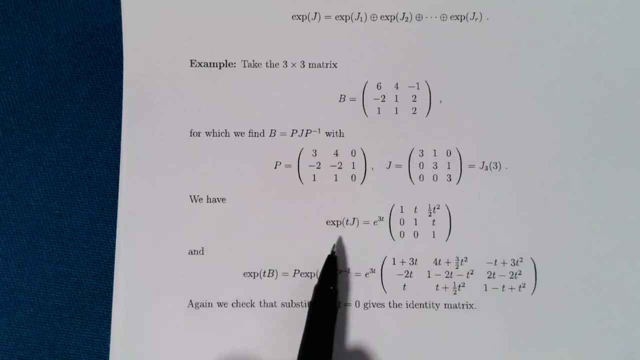 an earlier chapter. and so the exponential matrix e to the j t is e to the three t, one's down the matrix main diagonal, t's 1 on 2 factorial t squared, And finally, when you multiply it all out, you end up getting this rather complicated looking matrix here. 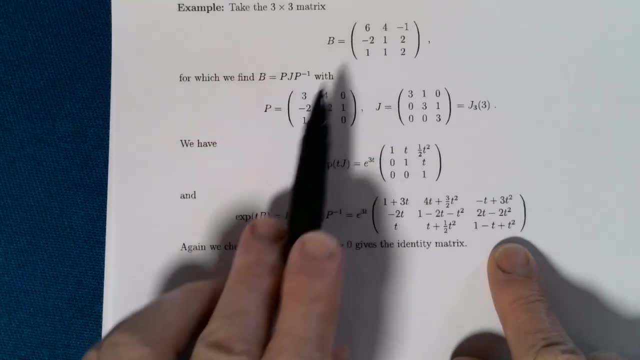 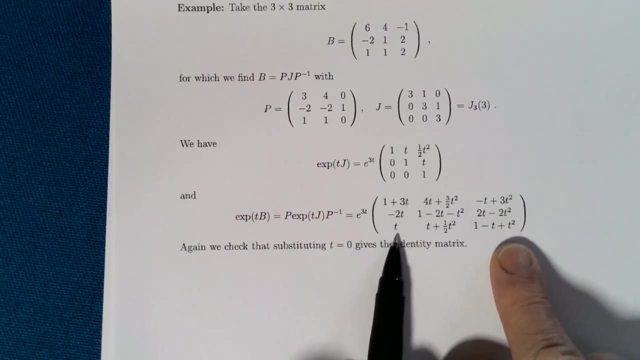 So this is p times, that's this p up here multiplied by this matrix. multiplied by the inverse of this matrix lands me to this one. here And again, we can at least check that it makes sense If you put t as 0,. 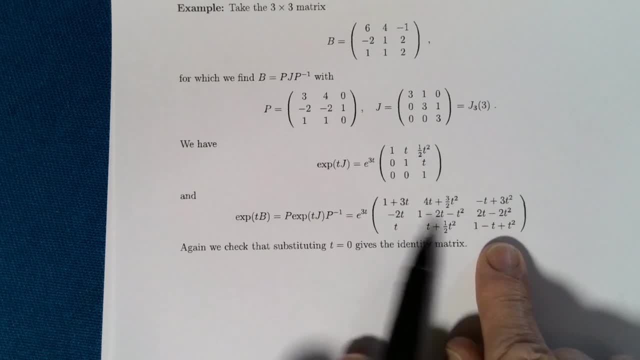 then all of the terms are 0,, except you get 1s on the main diagonal, And that would just simply give you, and you put t as 0, so that would give you the identity matrix, which is what you'd expect. 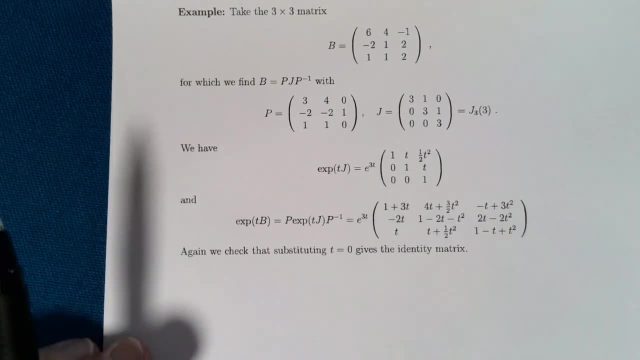 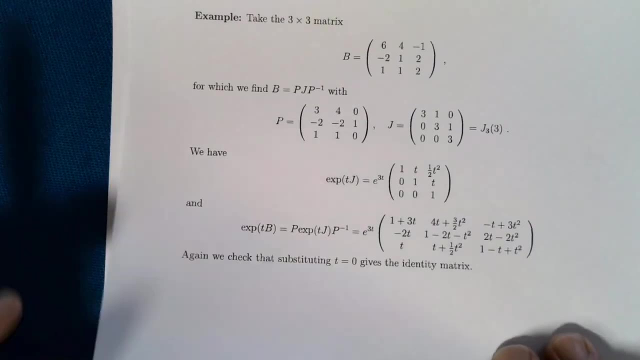 So that's what happens there. Now I wanted to go through a worked example of this, just to calculate how it works. You might like to try doing this yourself and then have a look. and have a look at what I've done here. 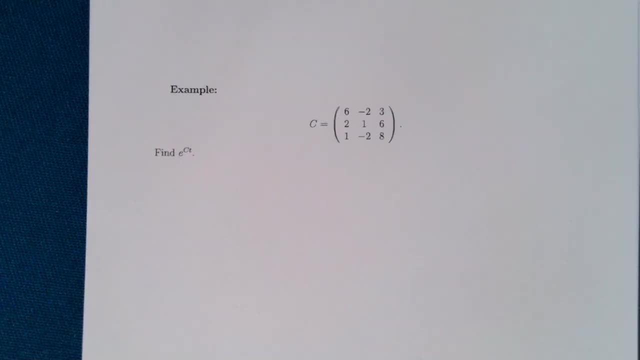 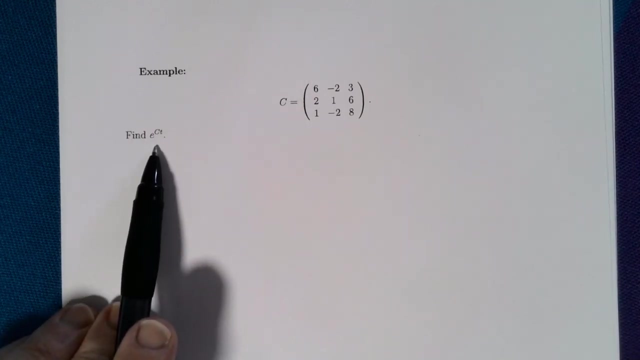 I'm going to show you, in fact, two ways of doing this particular one. So here's our matrix C. We want to find e to the ct. So if you're feeling confident, you might like to work this out yourself. 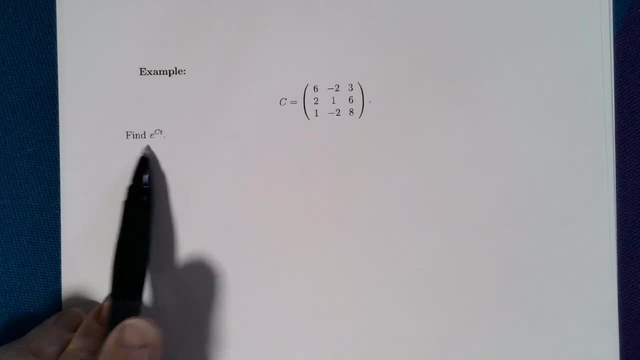 at this stage- and then double check- And here's the worked solution for this, And I'm going to do two ways of doing this. One is the long way and I'm going to show you a short way of doing it as well. 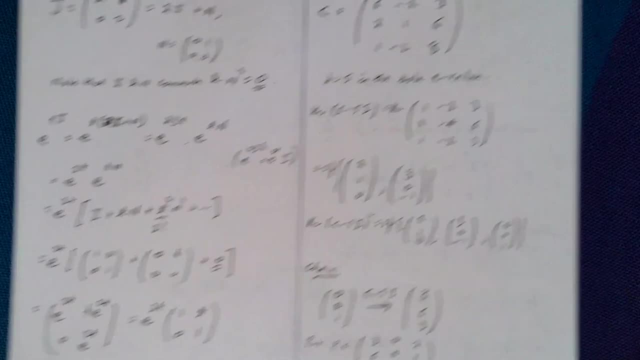 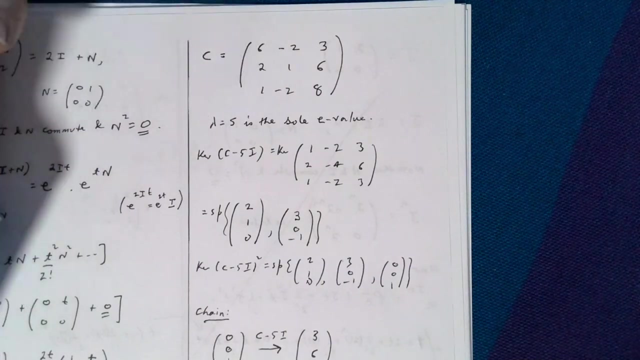 So here's the usual way. This is the usual thing we do. So here's our matrix C, And I tell you, it's only got one eigenvalue: lambda equals 5.. So in which case, from the trace. 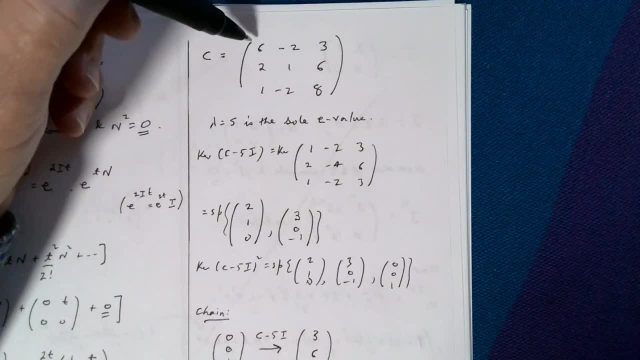 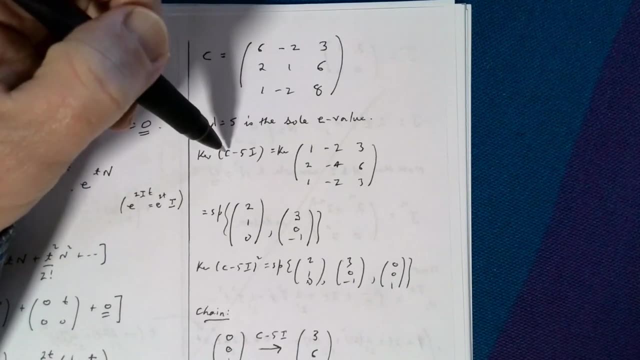 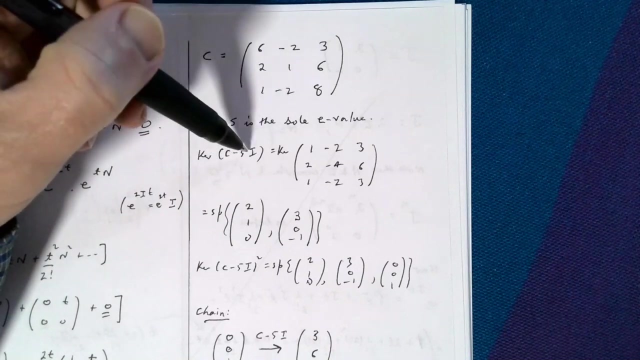 the trace is 15, so the eigenvalue has to be 5.. We work out the first kernel and we get this matrix. So this matrix, so the kernel of C minus 5i is the kernel of this matrix. And if you look at this, 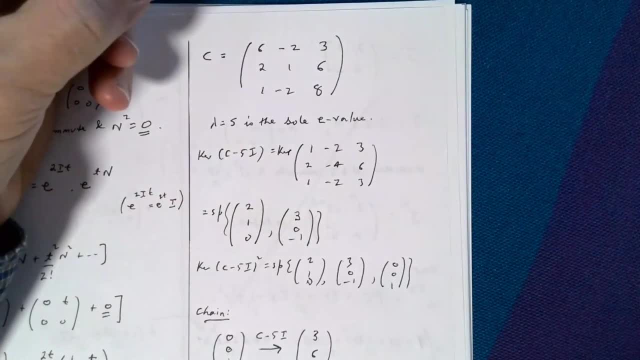 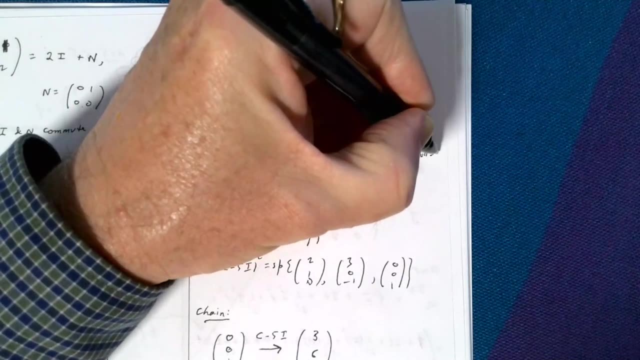 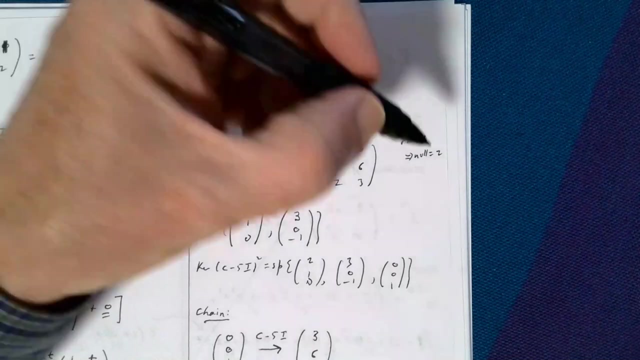 you'll see this has got rank 1,, nullity 2.. So the rank is 1, and that tells me the nullity is 2.. That means there are two eigenvectors hiding in here. So in terms of the onion that we had, 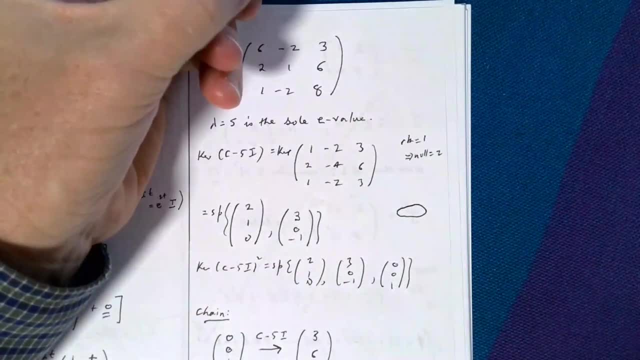 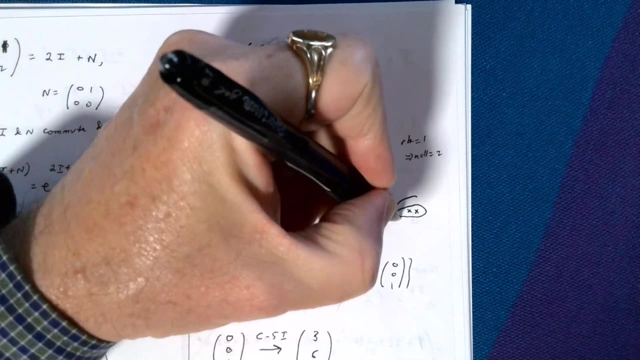 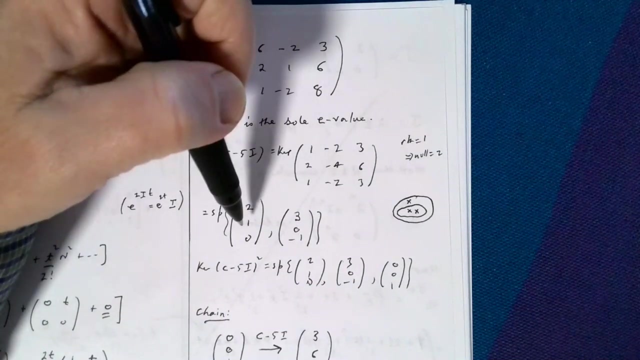 in an earlier chapter on Jordan forms. we've got two eigenvectors in here in the innermost kernel, and if we go to the next kernel out we're going to pick up one more generalized eigenvector. So the kernel of C minus 5i squared. 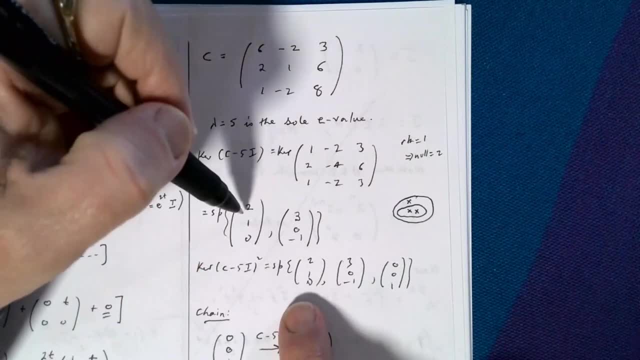 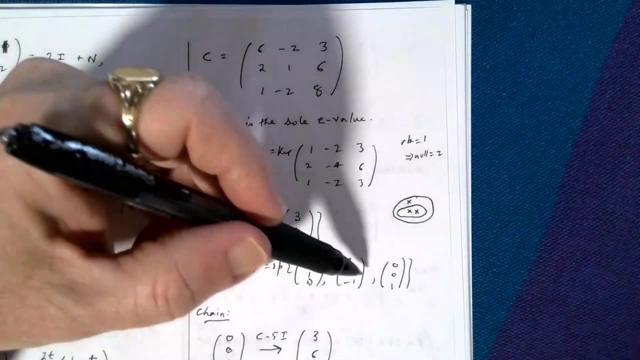 well, I always keep the two eigenvectors that I had. There they are, And then I toss in anything I like, really as long as it's linearly independent with these two. So I'm going to toss in 0,, 0,, 1.. 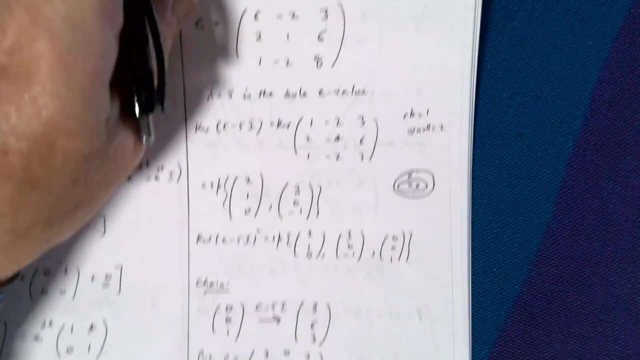 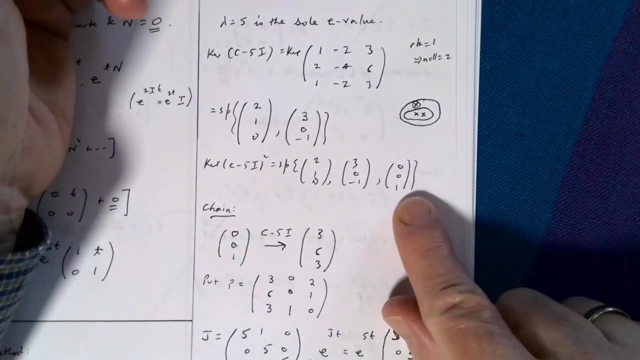 And we can build our P matrix then by taking a chain. So we're going to take our vector here, our generalized eigenvector 0,, 0,, 1, and we're going to chain in by multiplying by C minus 5i. 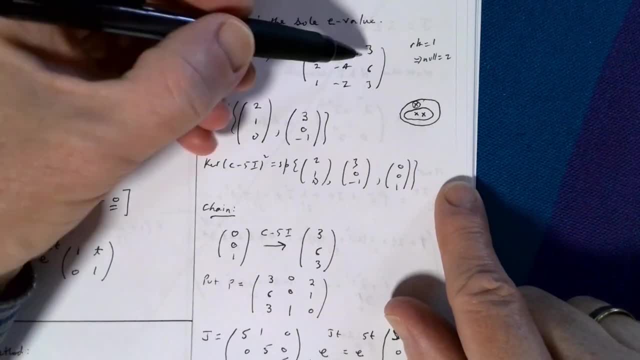 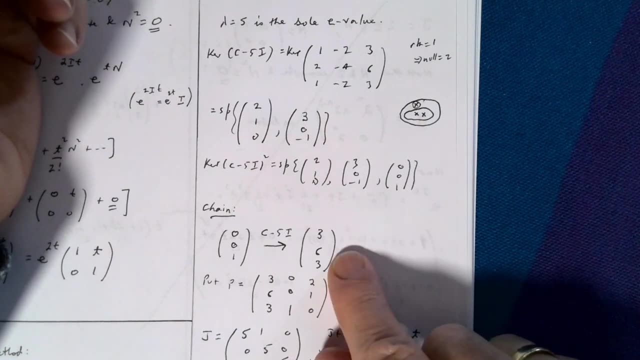 Now, that's just going to pull off the last column of this matrix up here, So it's just going to give me 3,, 6,, 3.. And we can check that this makes sense, because this must be. this is a vector somewhere in the eigenspace. 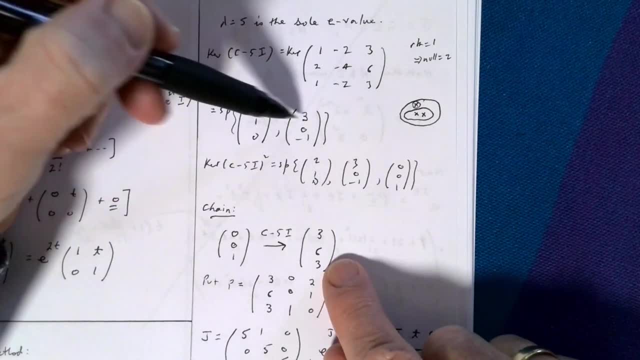 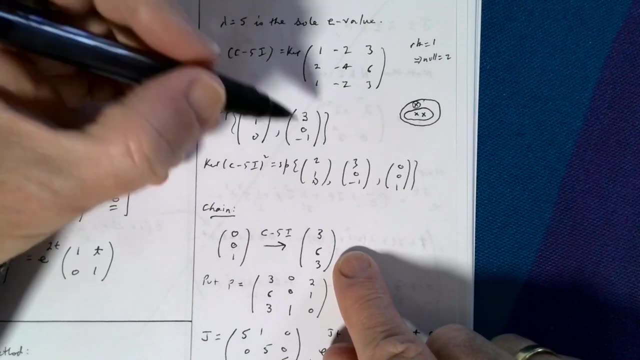 So this must be a linear combination of these two And indeed, if you take 6 of those minus 3 of those, you'll get this one. Okay, so it's 6 times this one minus 3 times that one. 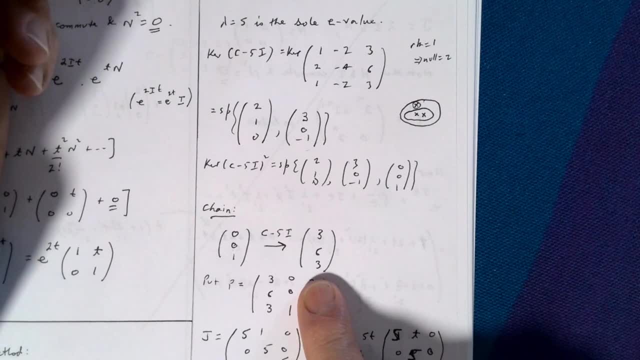 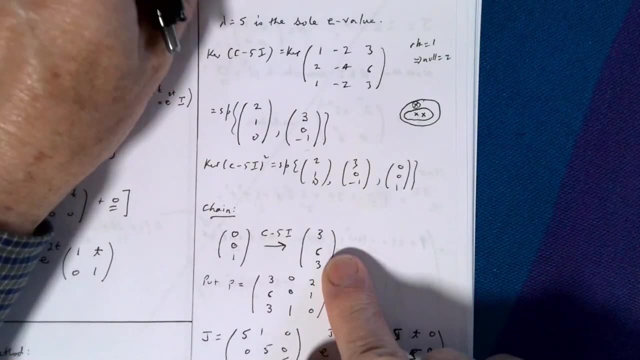 And that will give you this vector. So just double check that it is in fact in the eigenspace. So we put our P matrix, then We simply put in the chain. So I put. note the order again. 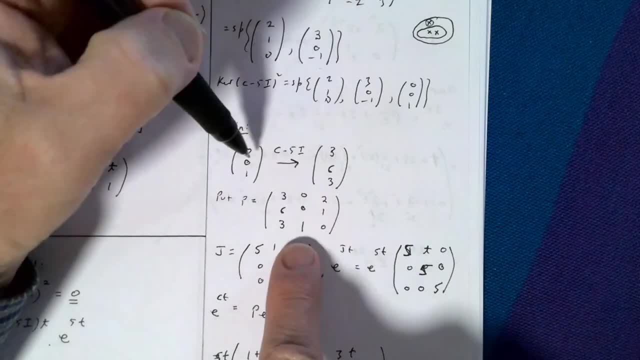 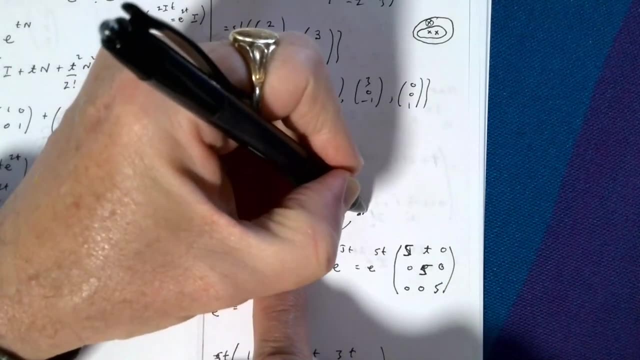 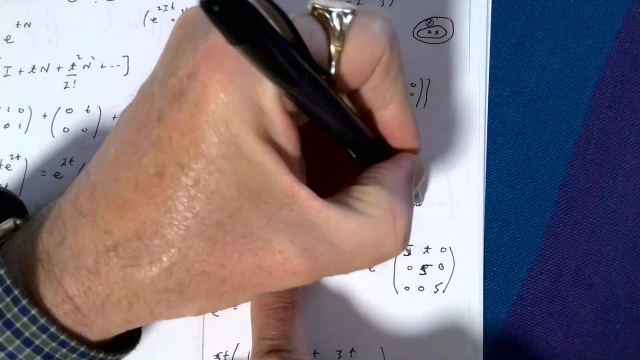 We put 3,, 6,, 3.. And then our generalized eigenvector, And we toss in here any other eigenvector, So any eigenvector that's not in the span, not in the span of the chain. 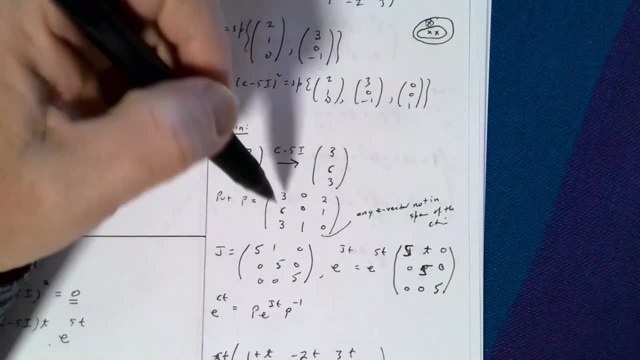 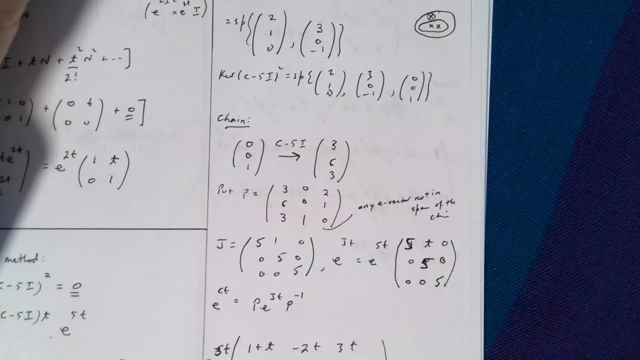 So we pick anything in here that's not in the span of these two. So that means this matrix- these will be linearly independent. So the matrix P has an inverse. So I just chose to put in the vector 2, 1, 0.. 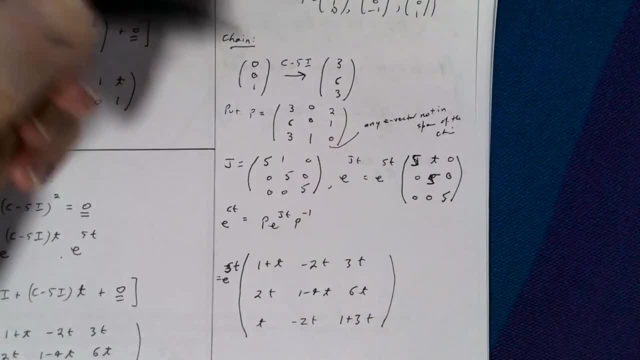 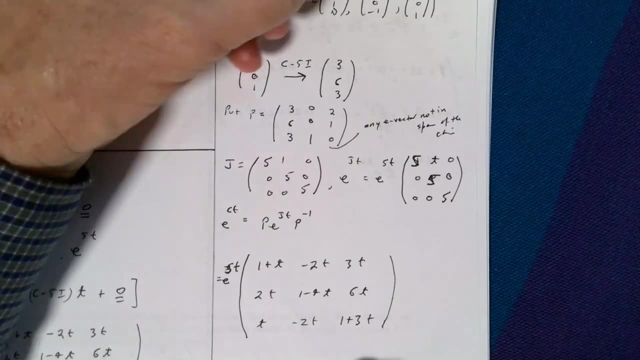 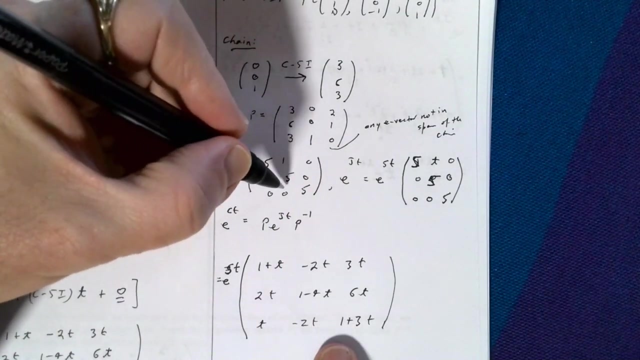 Now there's our J matrix then Now the J is going to have two blocks. So the J matrix is going to consist of a Jordan block of size 2. That's constructed by the chain, And then a Jordan block of size 1.. 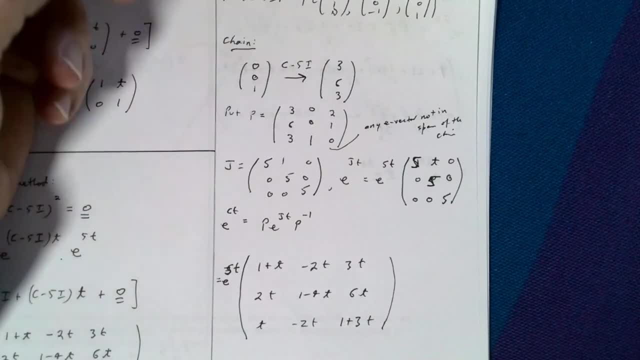 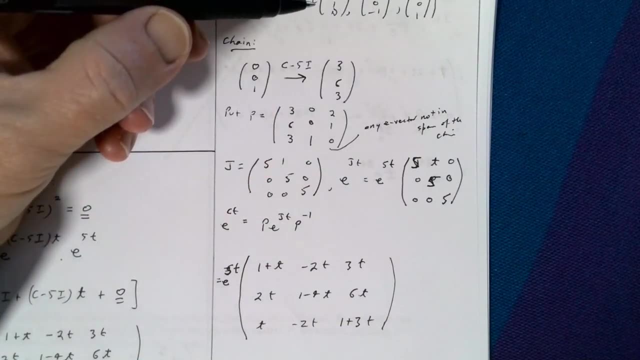 And that's constructed by the eigenvector. So E to the JT, then is E to the 5T times. we're just going to get 5s on the main, sorry, no, we're going to get 1s on the main diagonal. 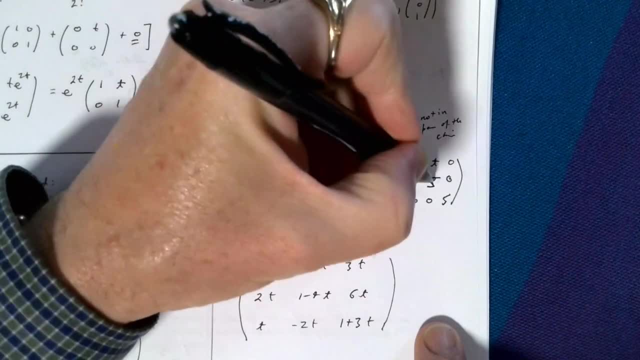 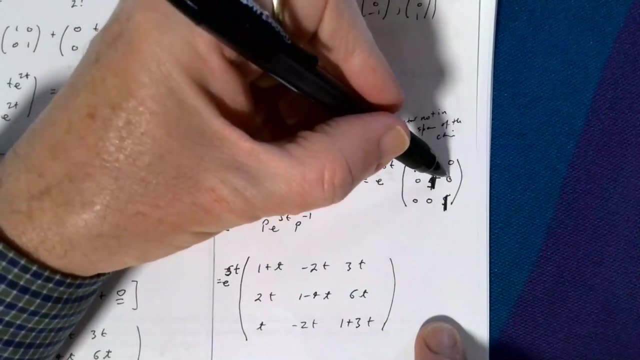 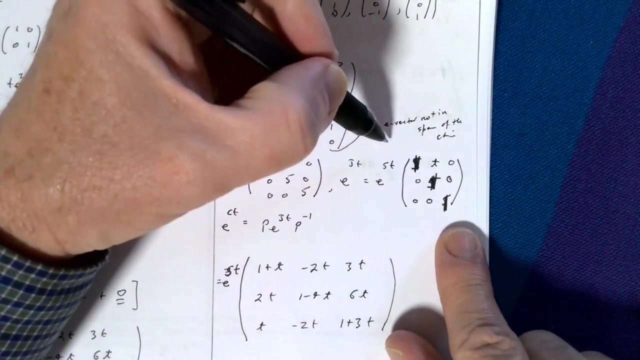 We're going to get 1s on the main diagonal and then a T up here and then 0s there. Sorry about that. So we're going to get E to the 5T times 1 on the main diagonal, And this block will give me a little T up here. 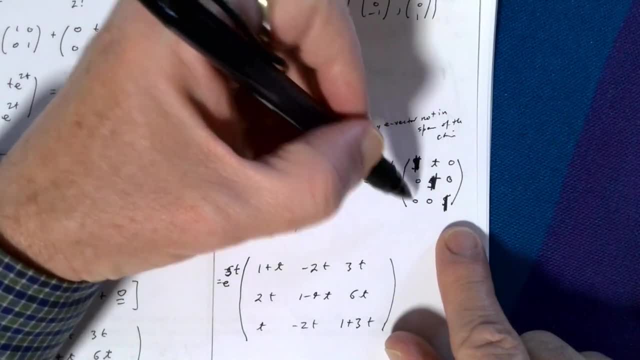 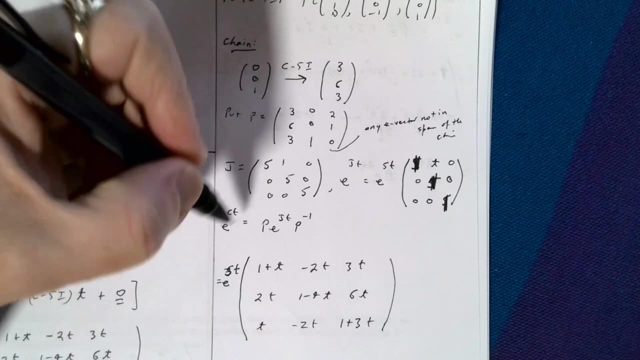 0s all around, And then I'm going to get an E to the 5T down here. So that's what we get, And if I work out, then either the CT is P or the JT is P inverse. 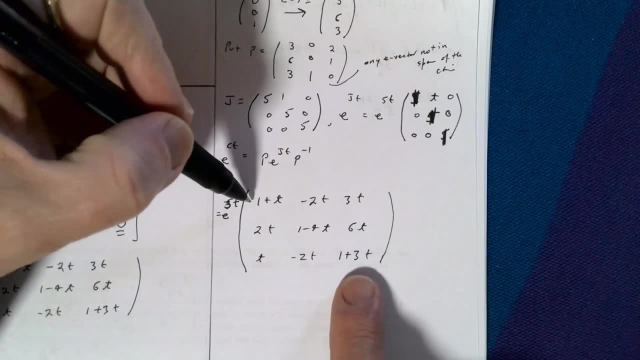 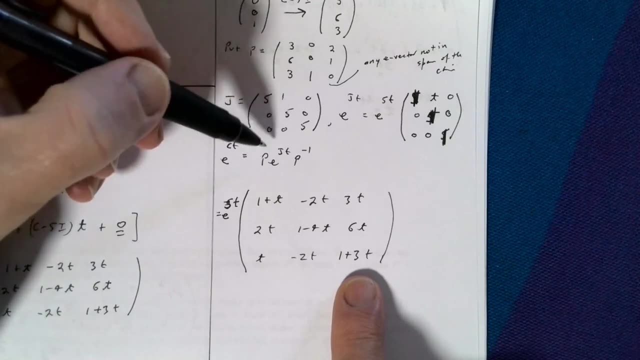 And if you multiply all that out you end up with this matrix here, And that takes a lot of work because you have to multiply P times this thing, But you've also got to calculate the inverse of this 3 by 3 matrix. 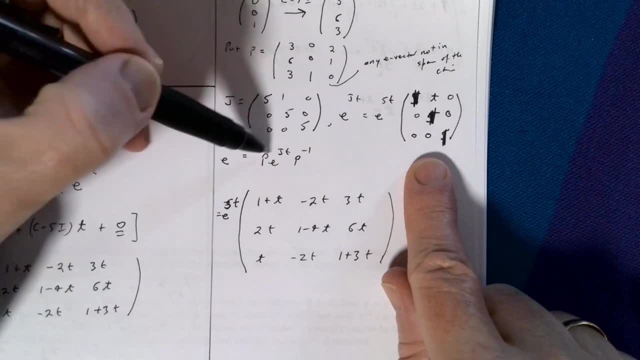 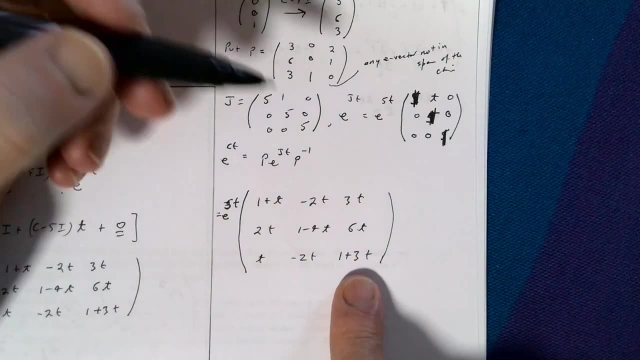 which takes a bit of work, And then multiply all that out And when you've done all that, that's what you end up with, And that's a lot of work. Again, we can check If you put T as 0,. 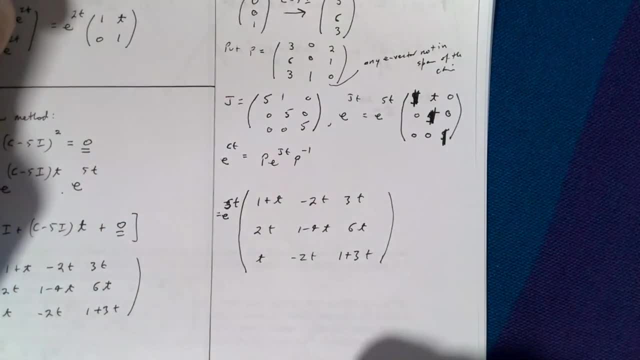 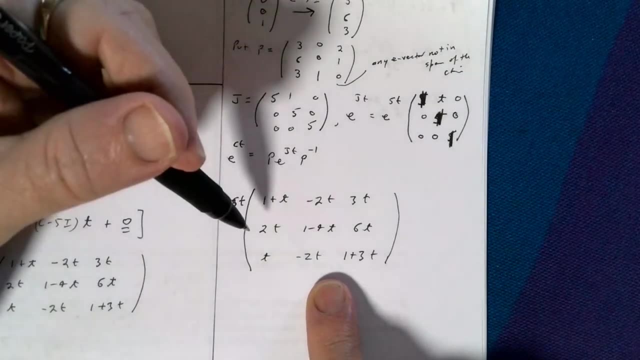 you'll get the identity matrix, So there must be, hopefully, an easier way. Well, in general, this is what you have to do, But there is a shortcut, which I'll mention here, which is a quicker method, And this relies. 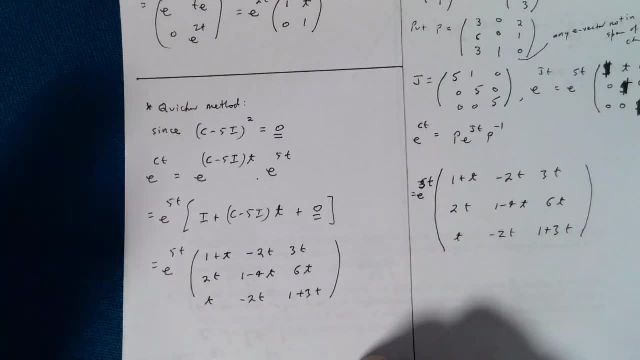 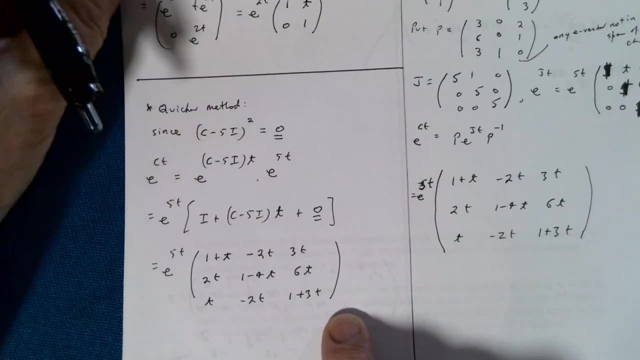 And this is a very useful idea. This is a quicker method And it relies on the fact that C minus 5I squared, is the zero matrix. So if you look back to the onion, we had two eigenvectors. We've got one generalized eigenvector. 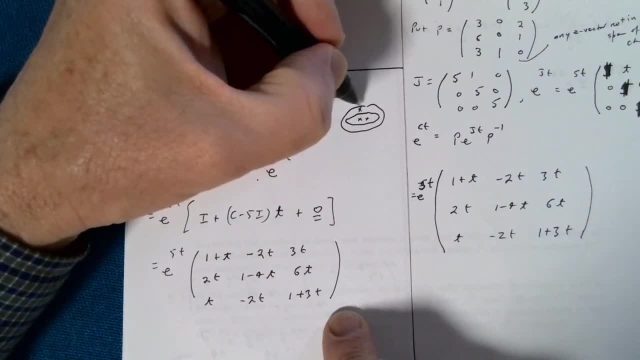 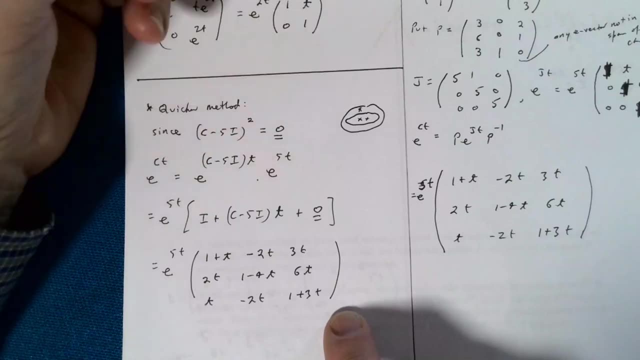 So this is the kernel. This represents This space. here is the kernel of A minus 5I squared And it's got nullity 3, so therefore rank 0.. So C minus 5I squared is the zero matrix. 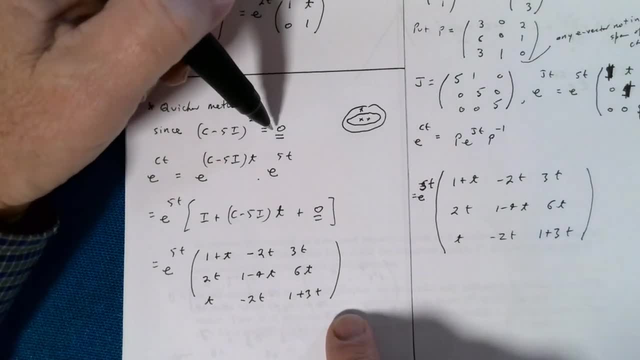 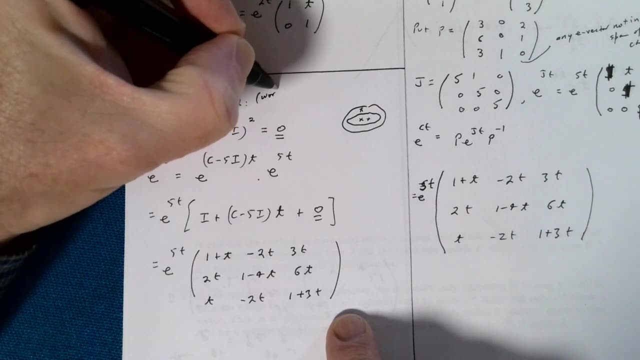 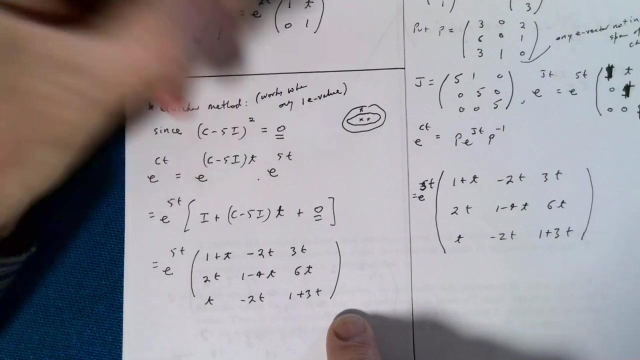 Now, this only works because we only have one eigenvalue. This method only works for one eigenvalue. It works when there's only one eigenvalue. If you've got more than one, then sorry, you've got to use this other method over here. 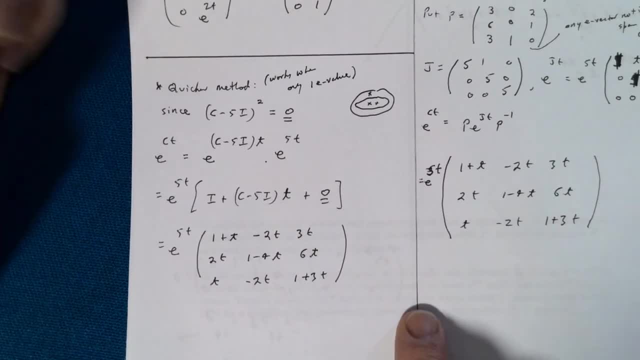 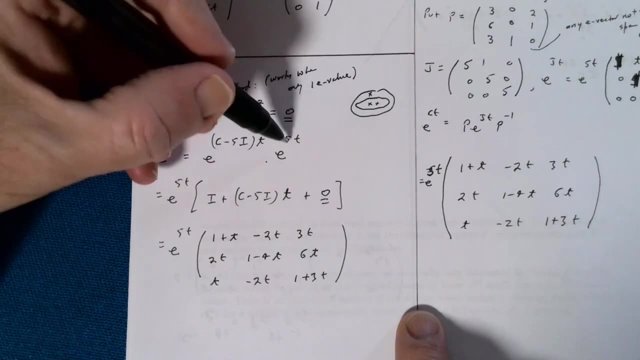 that takes a lot more work. So E to the Ct. Well, I just simply write this as C minus 5It, And then I'm really writing E to the 5Ti. As we've seen, E to the 5Ti is I times E to the 5T. 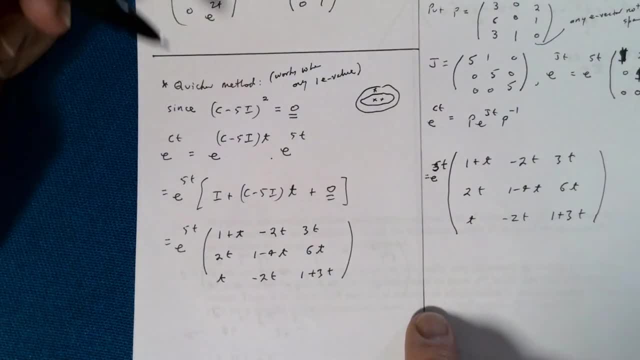 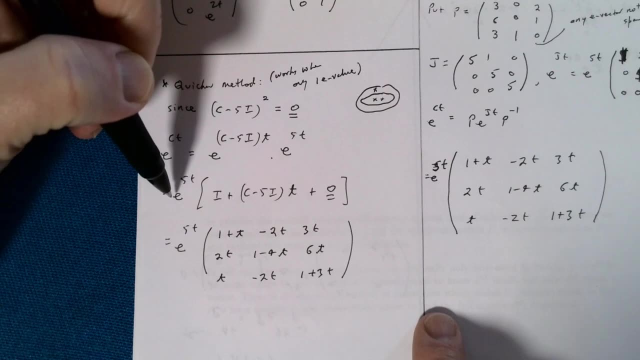 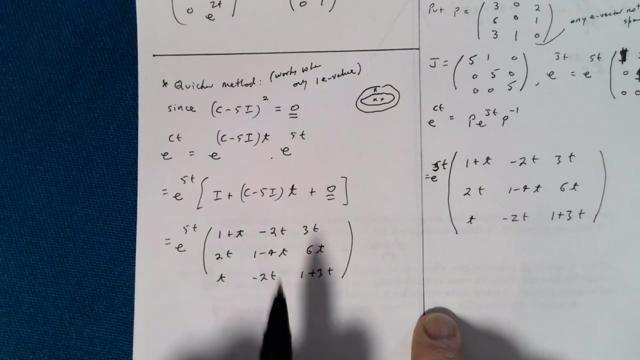 So just note that step there. And we can do this simply because I is the identity matrix. It commutes with everything. So this is E to the 5Ti, And now I can expand this out in series, So I just get the identity plus C minus 5It. 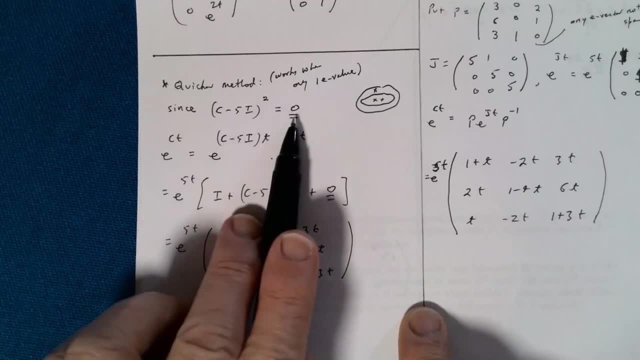 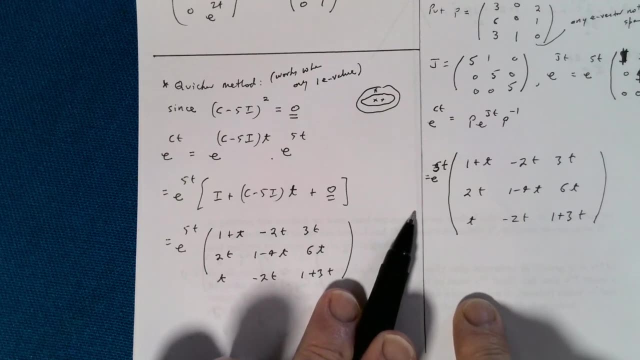 And when I take the next power up, I'm just going to get the zero matrix, And so all of the remaining terms here are all just lists of zero matrices And then, and so I just end up with this And there it is. 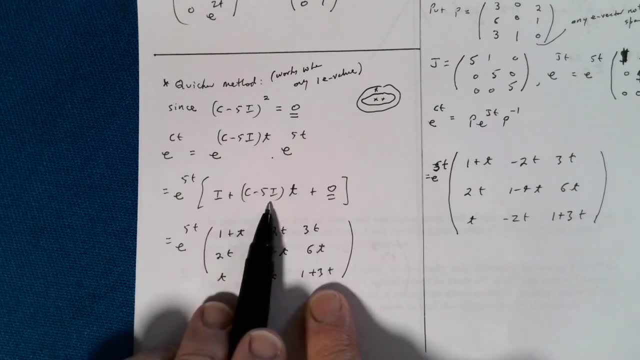 And so I simply write down C minus 5It. We worked that matrix out before. That was over the other side- And I simply multiply that matrix by T and then combine it with the identity, And that's what we end up with. 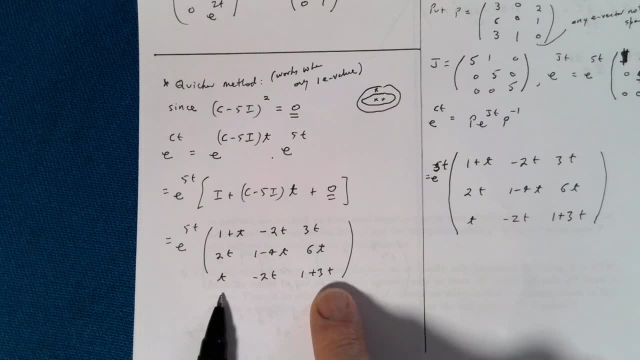 And that, of course. that, of course is in fact, where I got the answer over here from. I didn't actually work out P inverse. I used this fact that that's what the answer had to be. So that's a shorter method, a much quicker method.